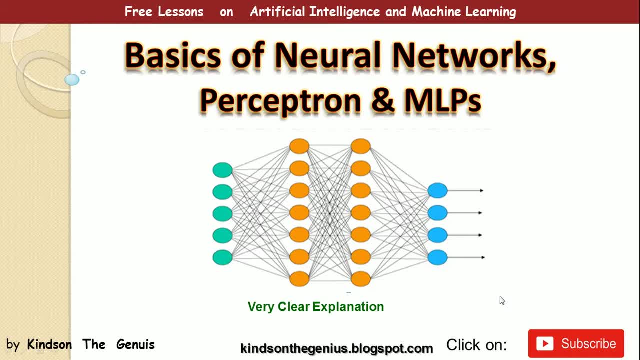 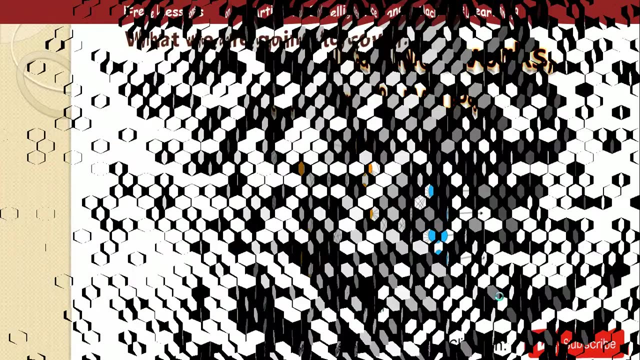 because my videos are based on requests. So if you request a video or you request a tutorial or a lesson, I'm going to make that video for you, But that will be for my subscribers. So please click on the subscribe button to subscribe at this point. Alright, so what? 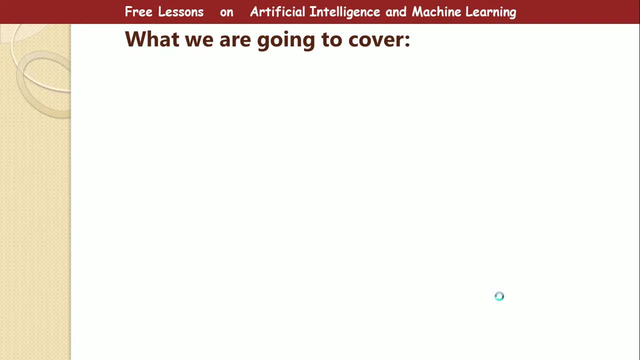 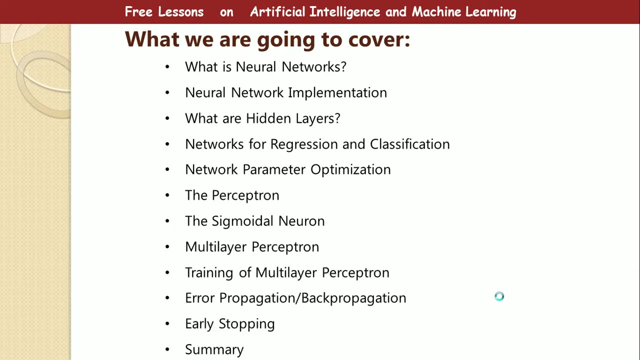 are we going to cover today? Today, in about 10 to 15 minutes, we are going to cover the following topics: What is neural network? Neural network implementation. What are hidden layers? Networks for regression and classification, Network parameter optimization, The perceptron, the sigmoidal neuron. Multi-layer. 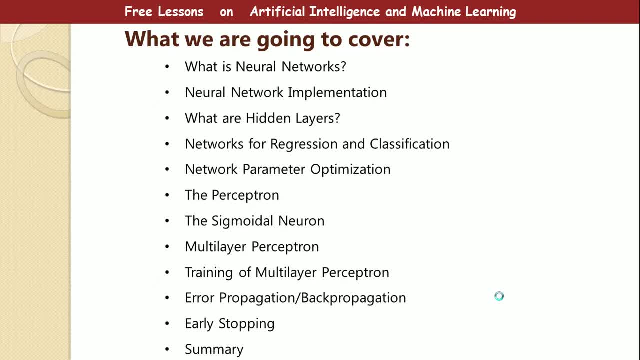 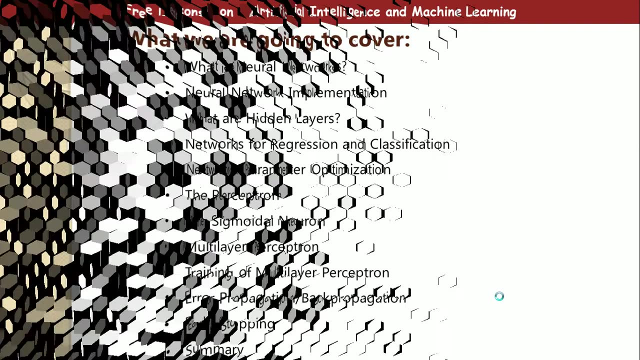 perceptron, Training of multi-layer perceptron, Error propagation and back propagation, Early stopping, and we summarize what we've learned. Alright, so in about 10 to 15 minutes we are going to cover all of these topics. So let's start with the first one. What is a neural network? As you can see, a neural network. 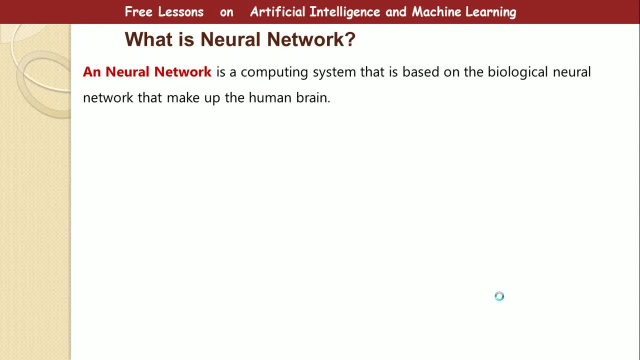 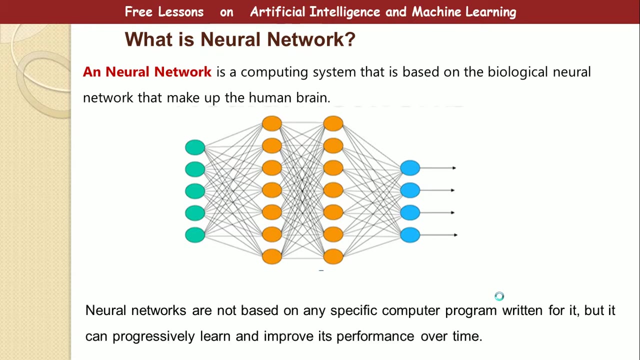 is a computing system based on the biological neural network that make up the human brain. So basically, a neural network is a subcomponent of an artificial intelligence system that tries to mimic how the human brain works. Neural networks are not based on any specific computer programs written for it, but can. 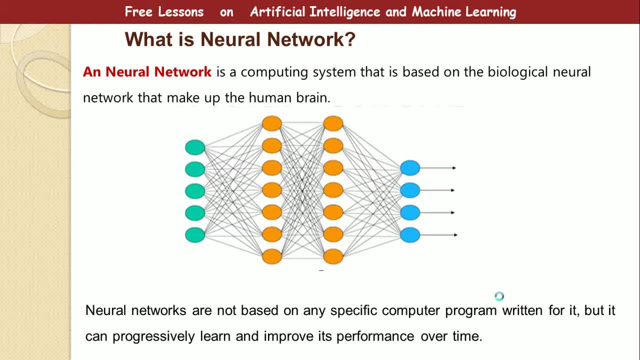 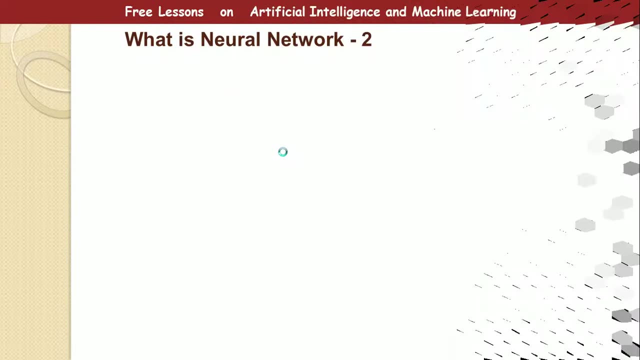 progressively learn and improve its performance over time. So the diagram you see here is an example of a neural network made up of connections and made up of nodes. Alright, so what is a neural network? Let's give more explanation. So what you see here? is a neural network made up of cells. Alright, so what is a neural network? Let's give more explanation. So what you see here is a neural network made up of cells. Alright, so what you see here is a neural network made up of cells. 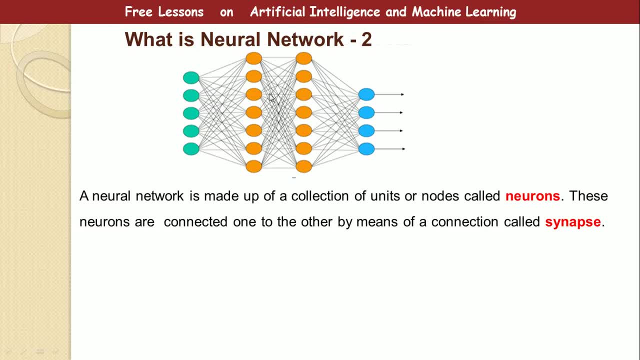 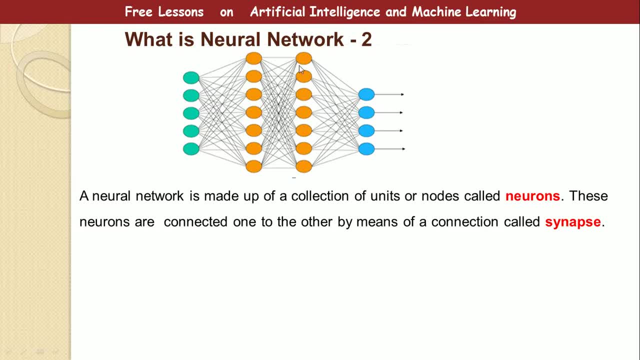 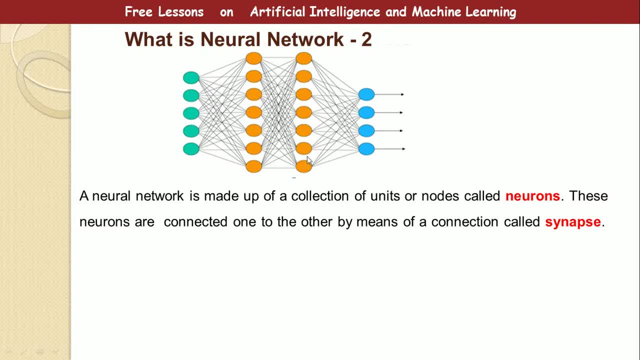 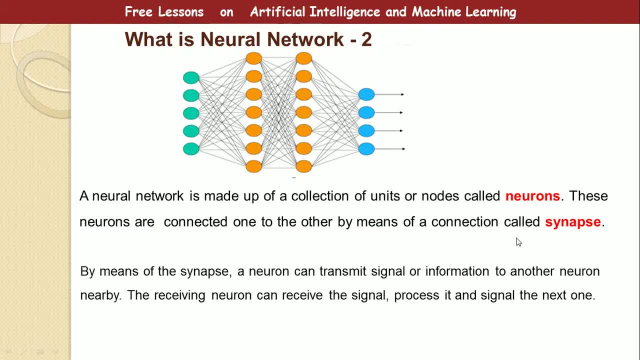 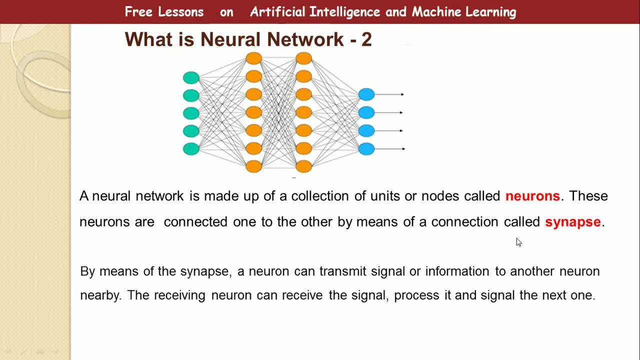 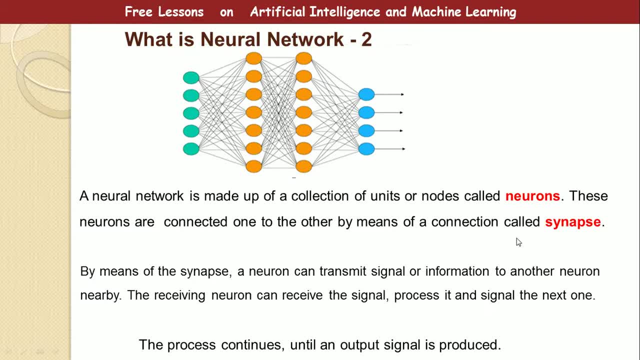 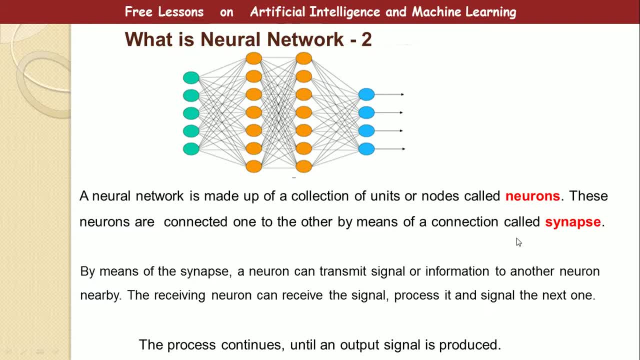 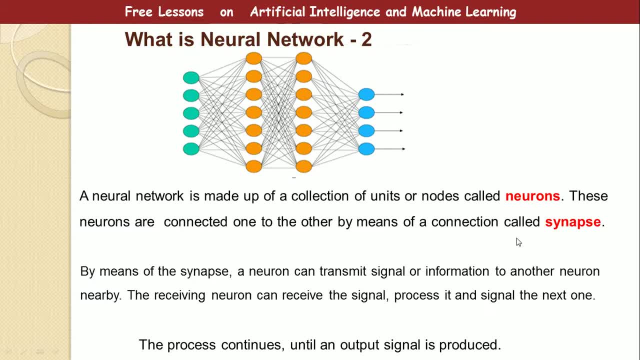 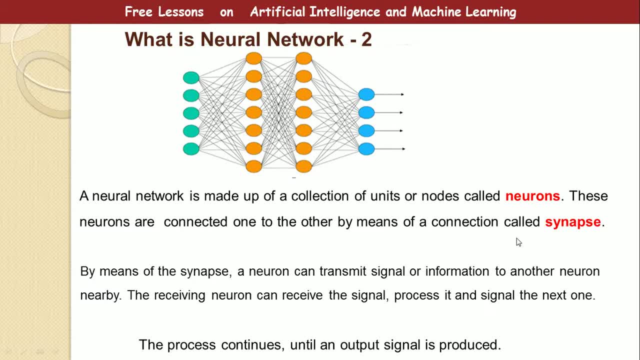 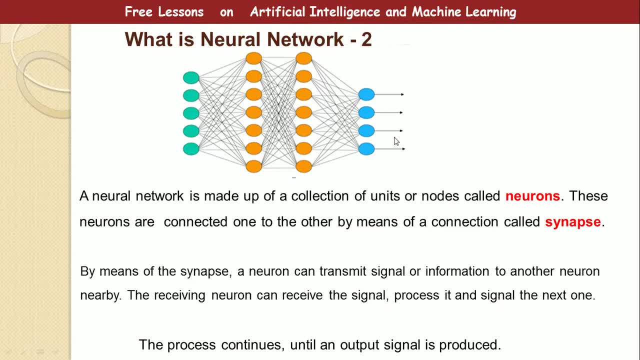 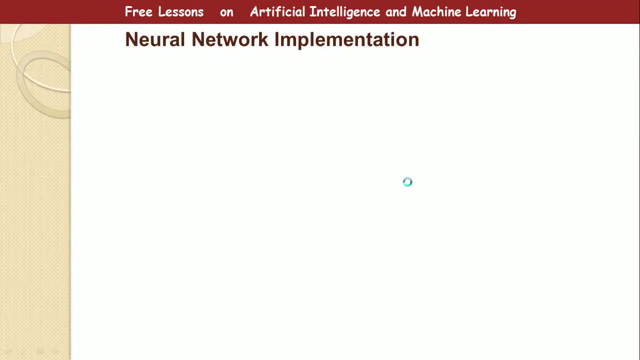 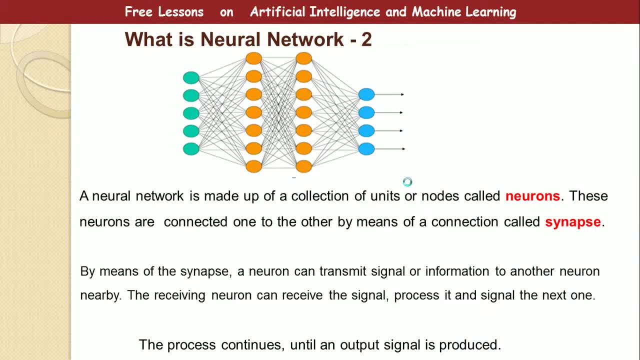 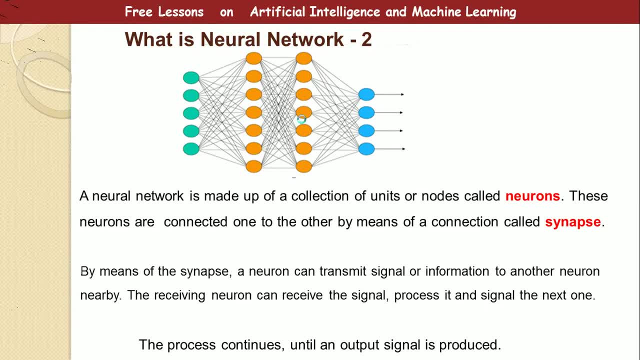 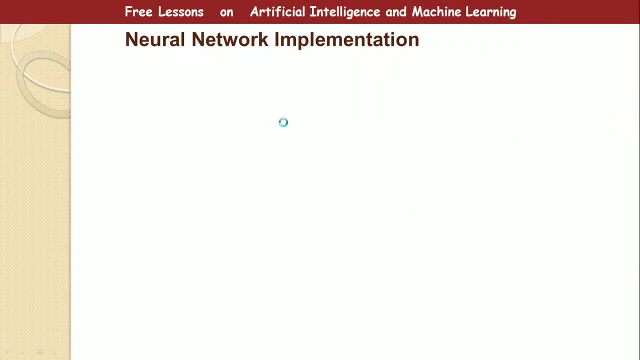 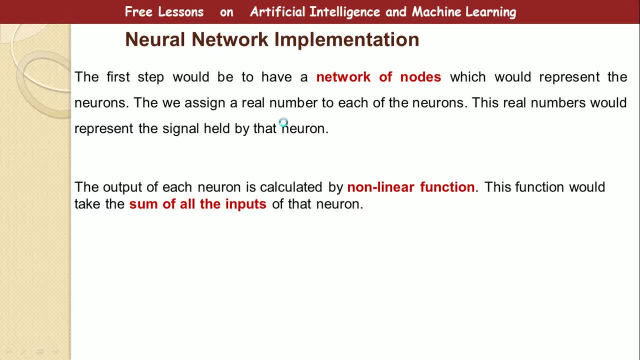 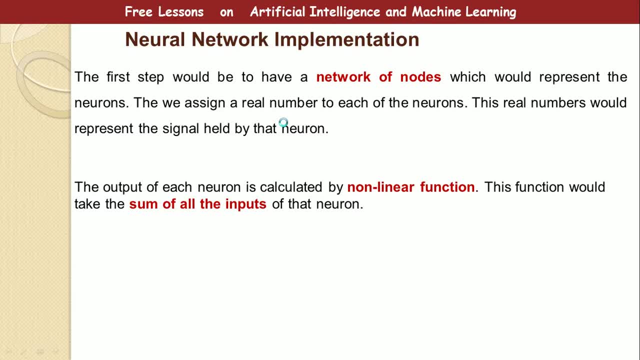 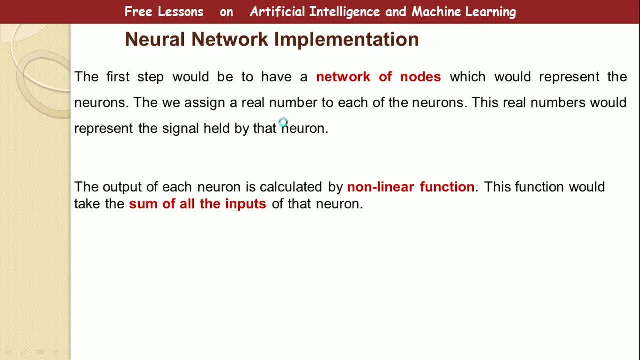 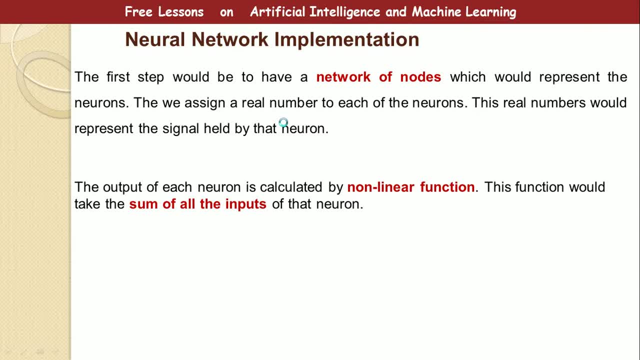 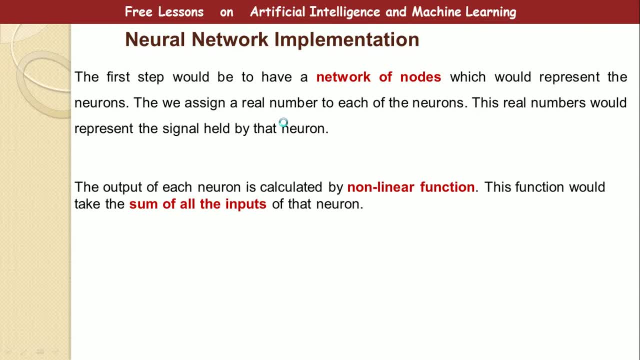 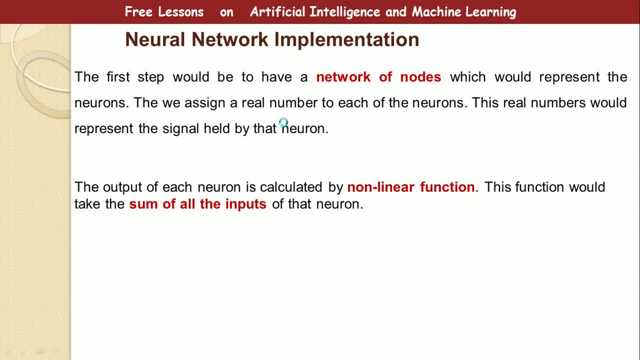 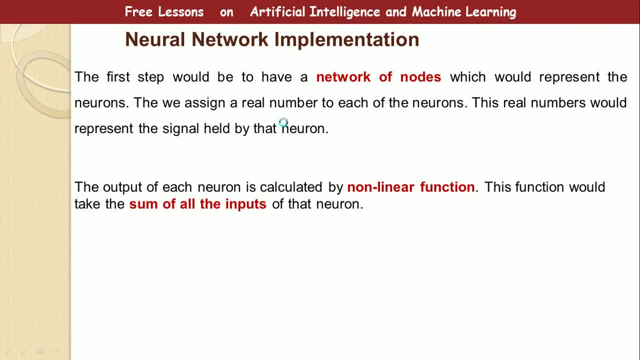 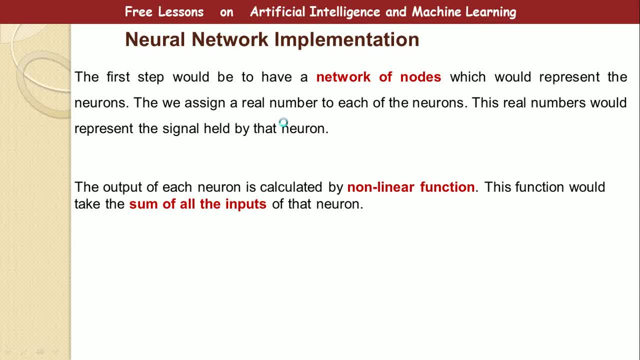 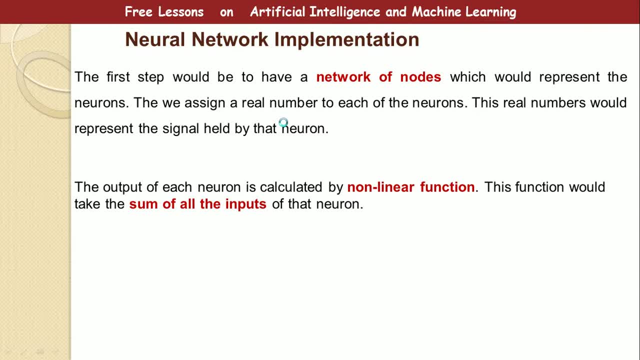 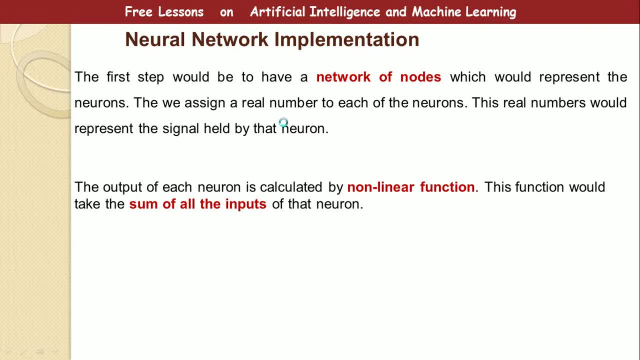 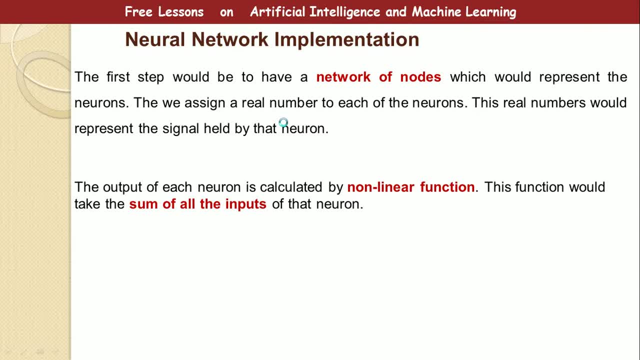 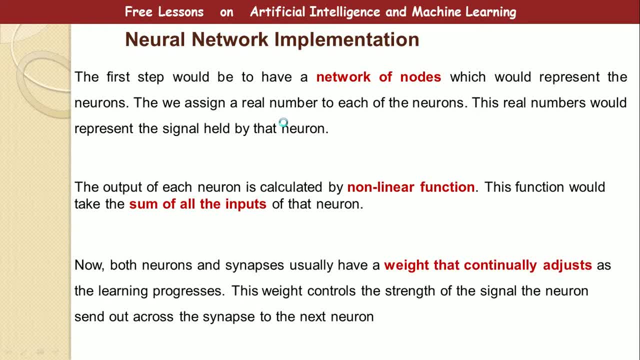 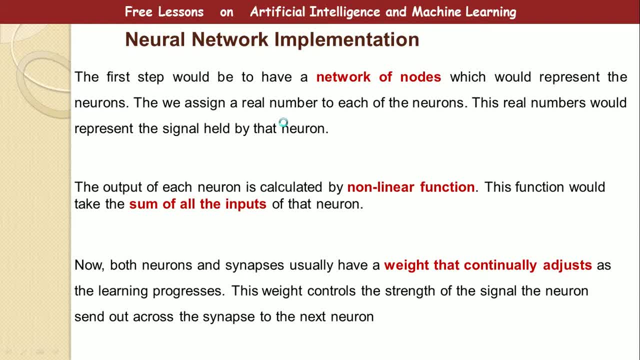 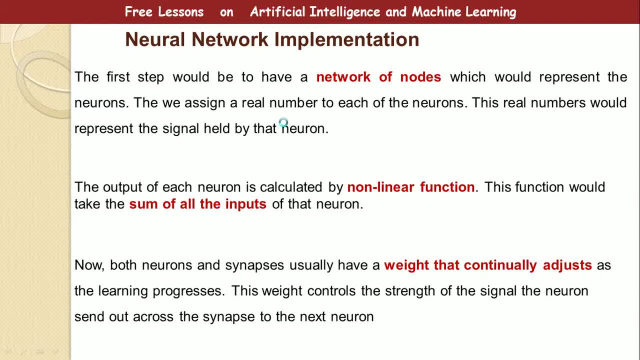 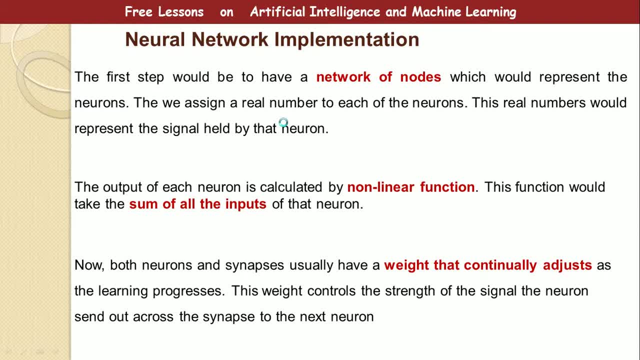 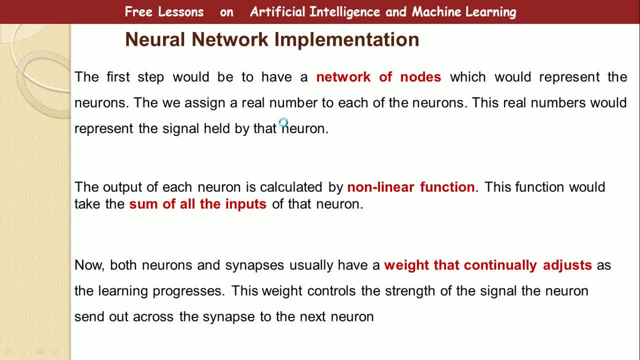 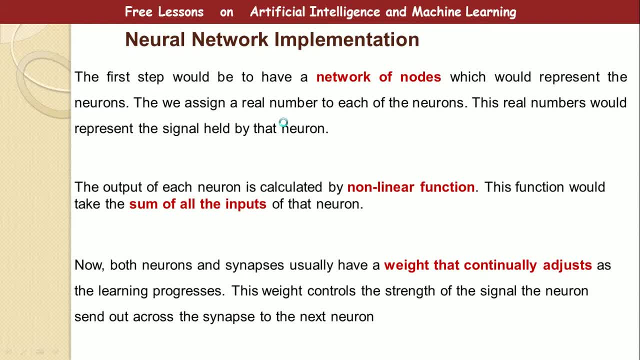 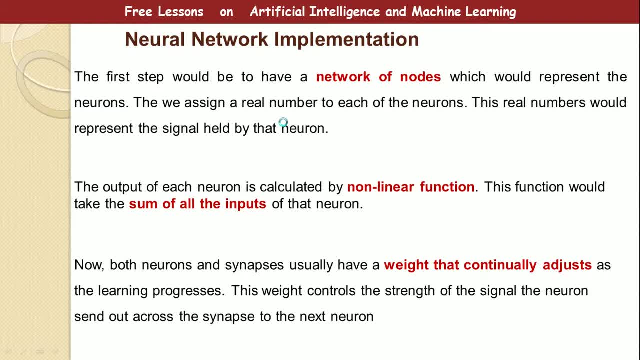 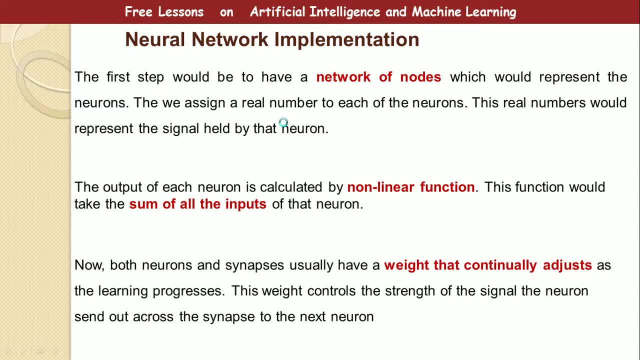 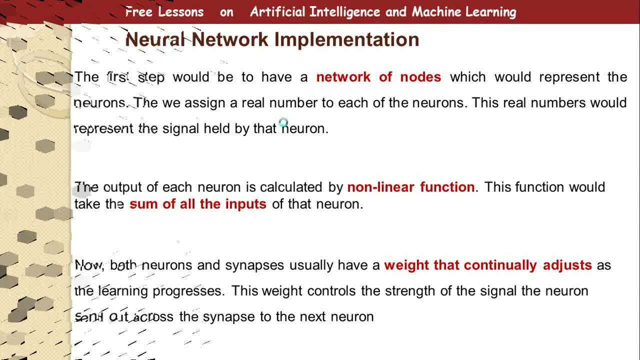 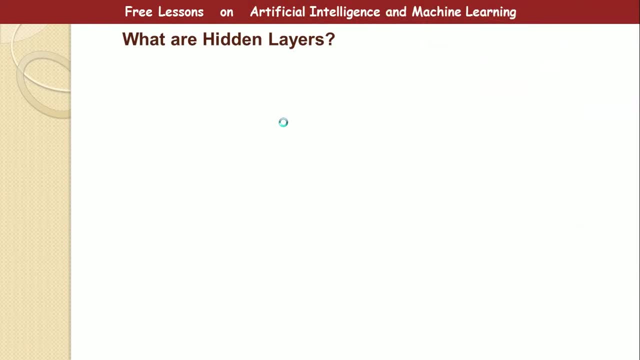 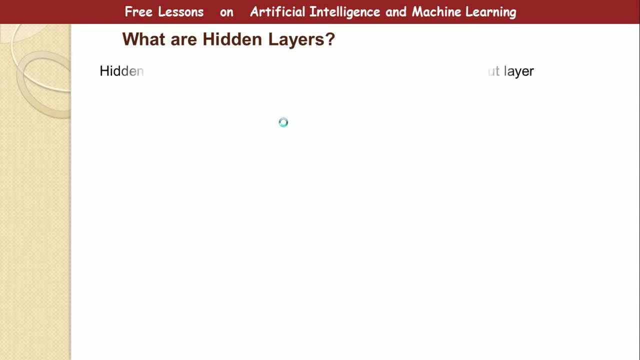 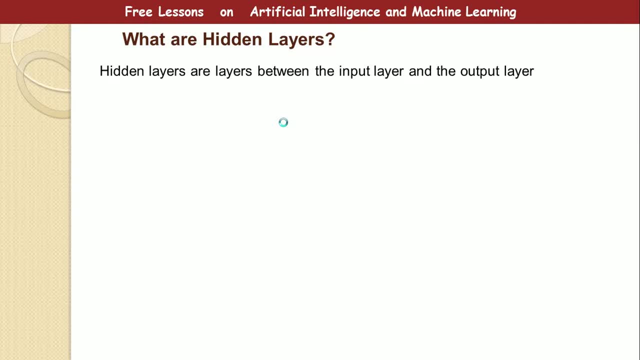 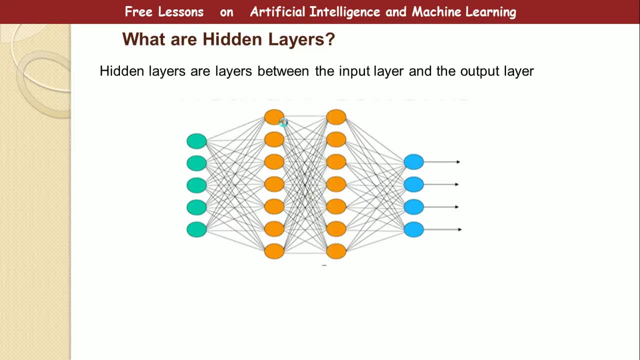 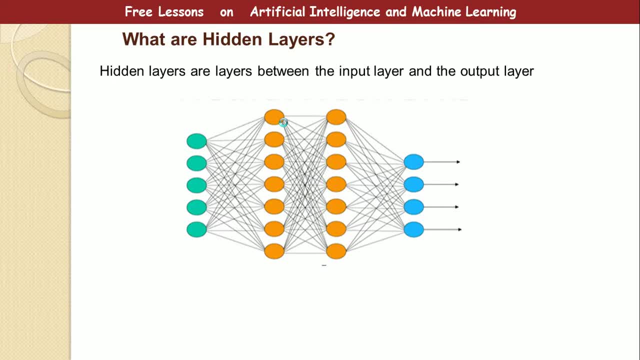 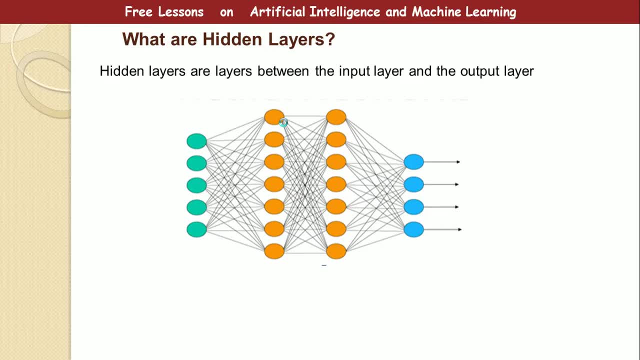 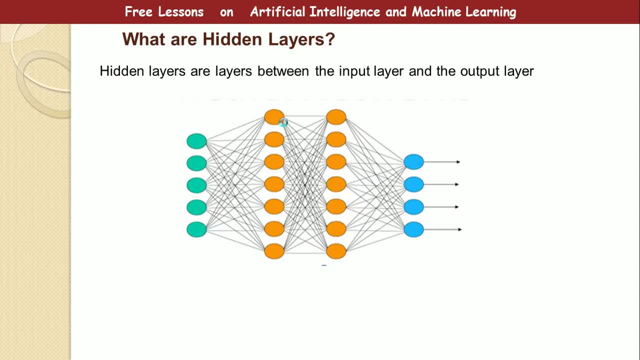 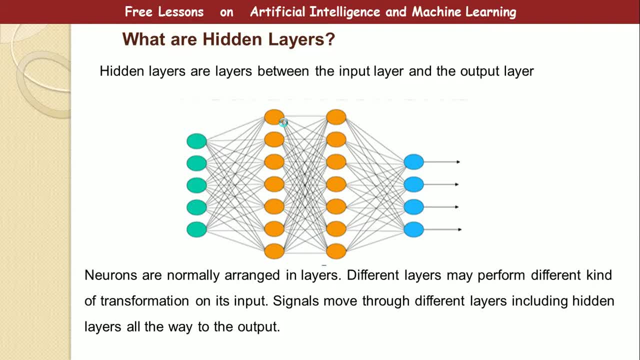 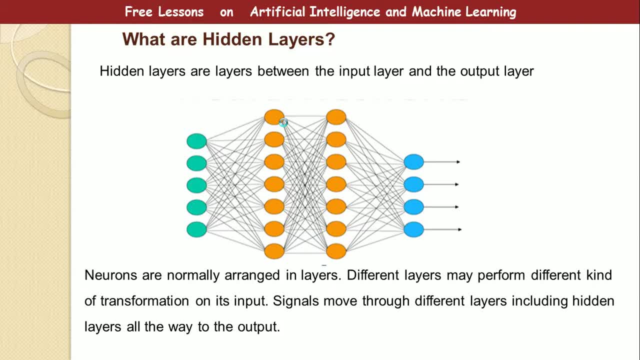 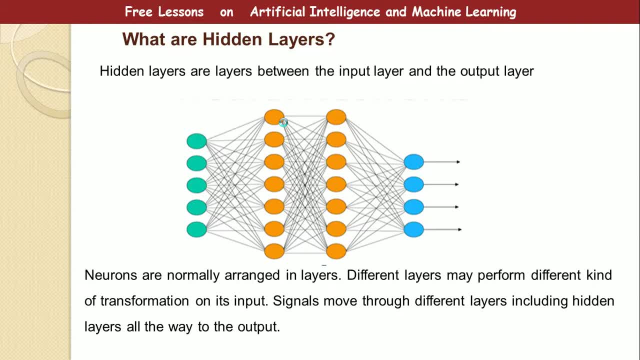 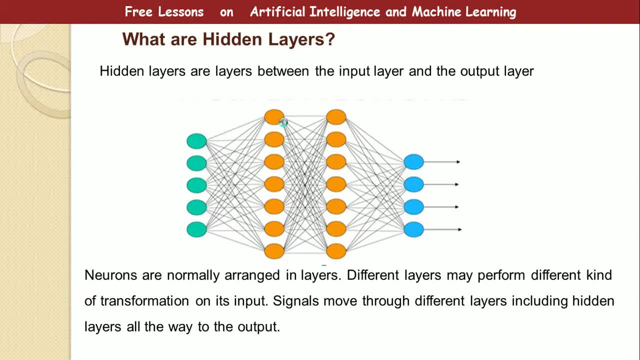 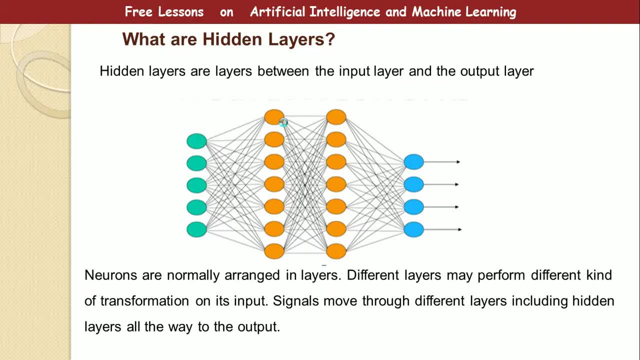 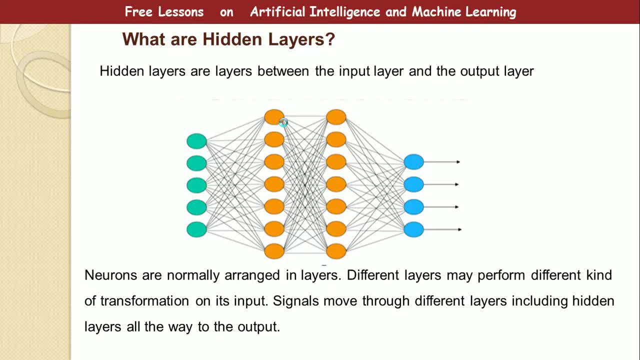 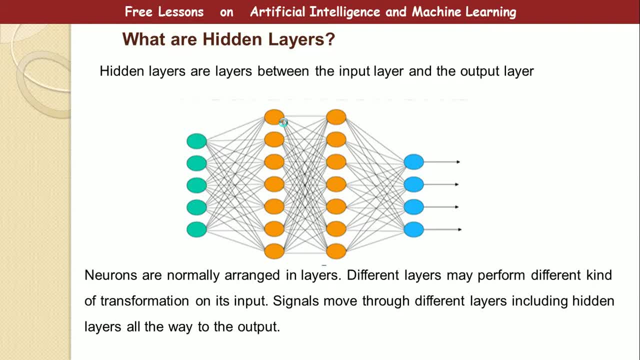 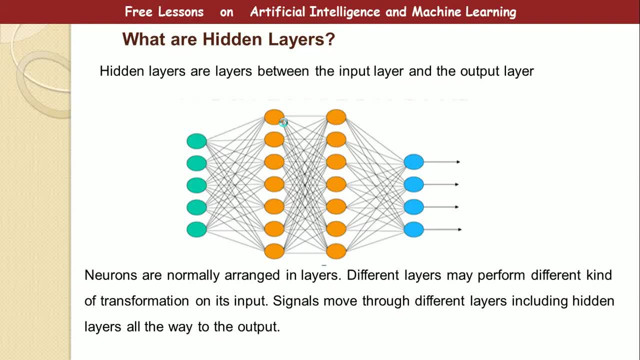 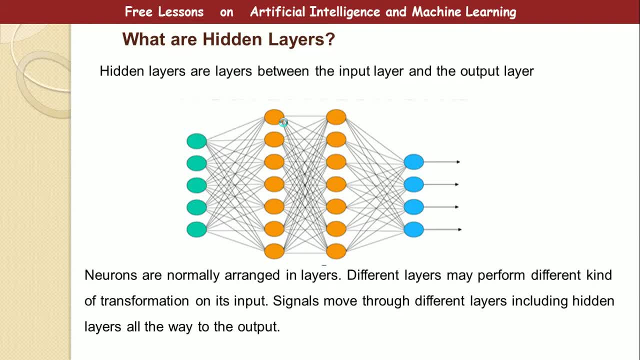 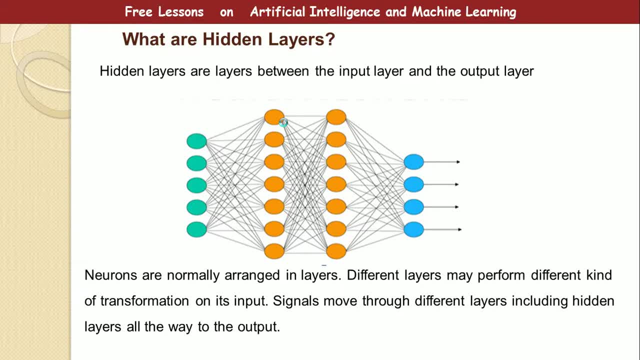 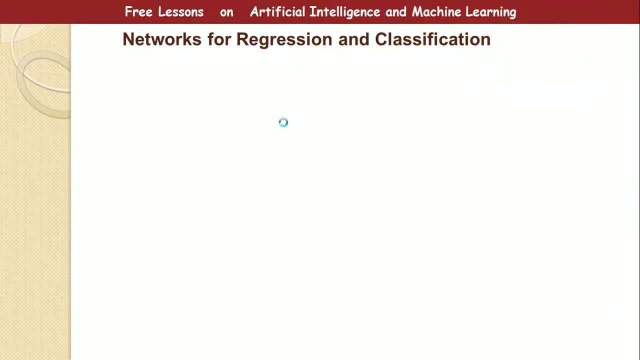 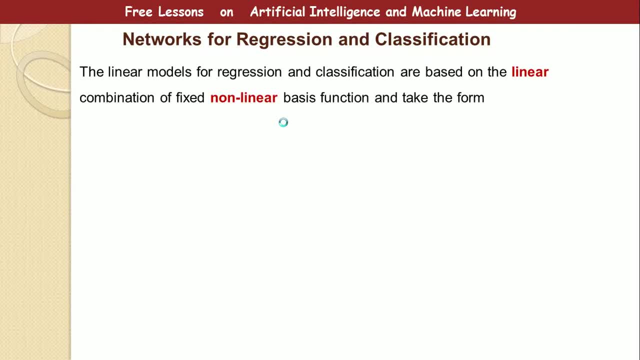 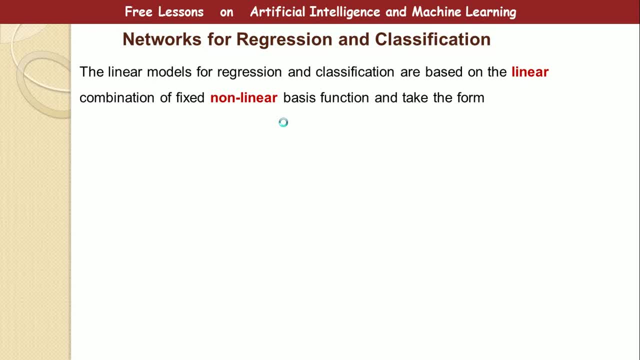 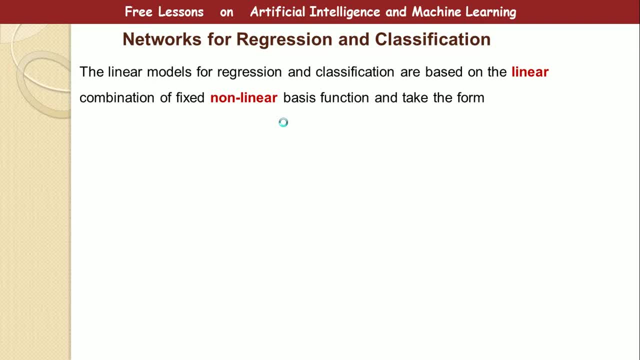 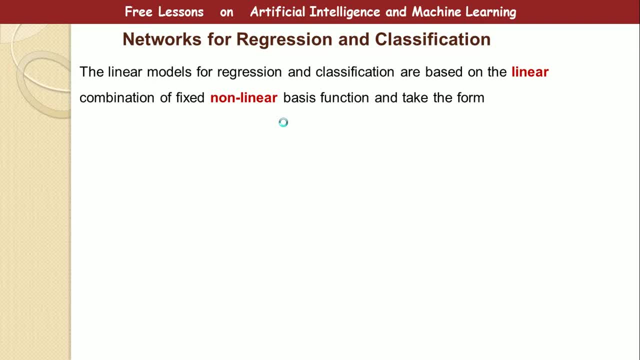 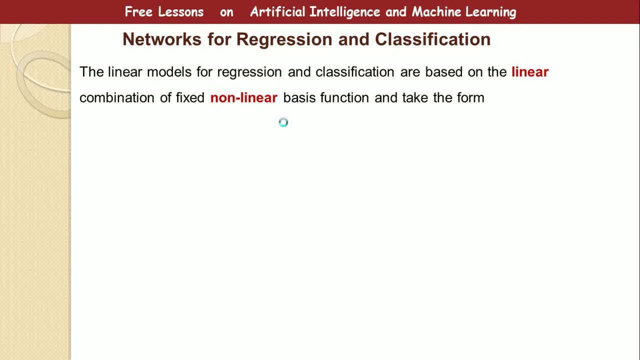 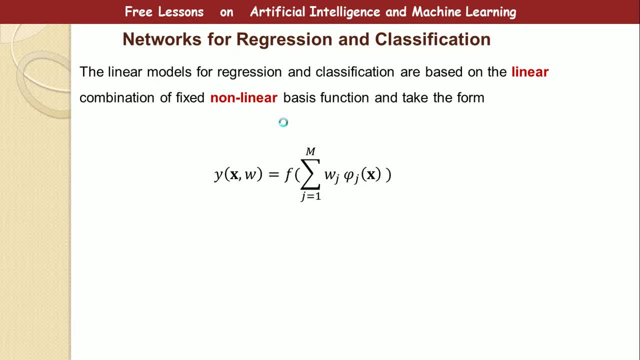 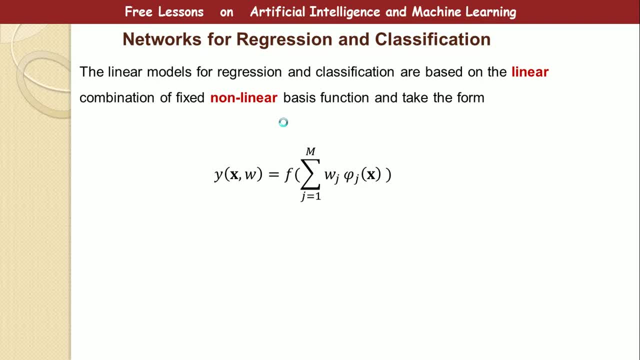 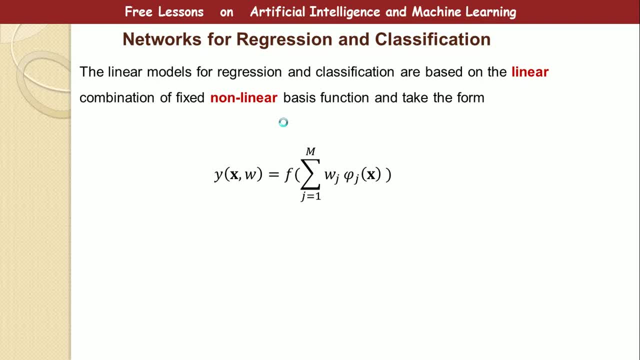 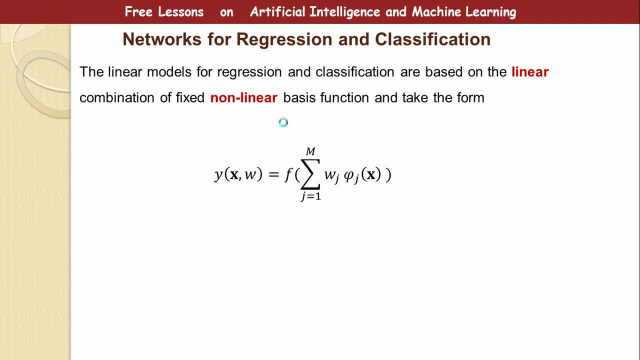 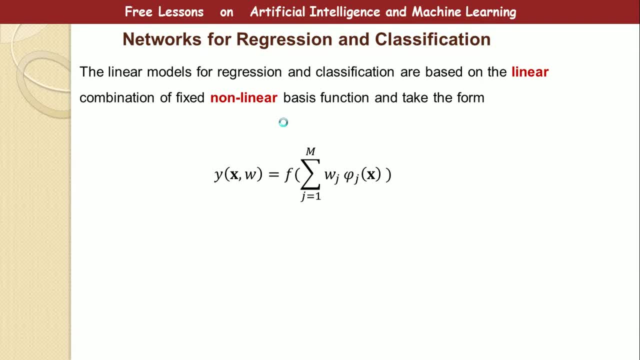 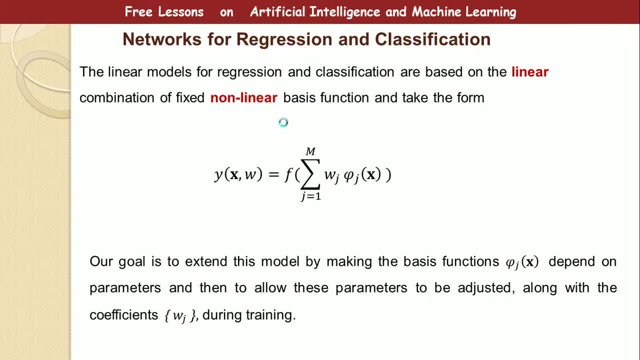 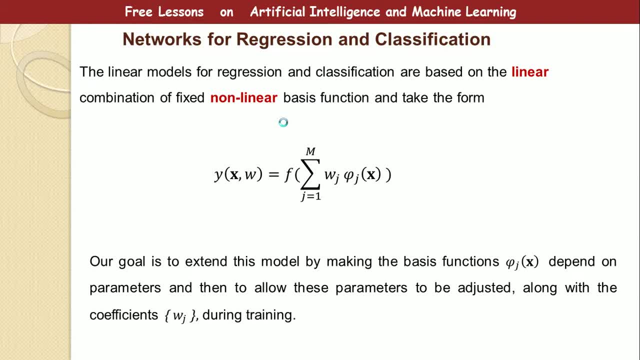 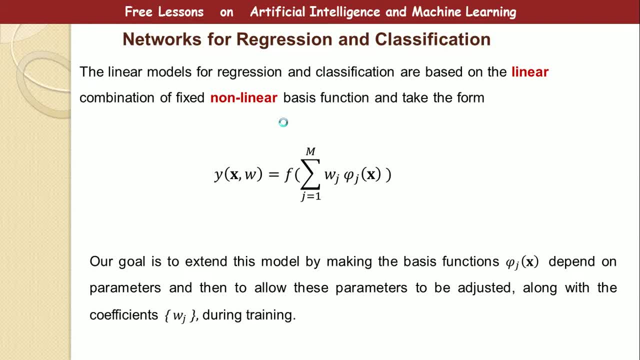 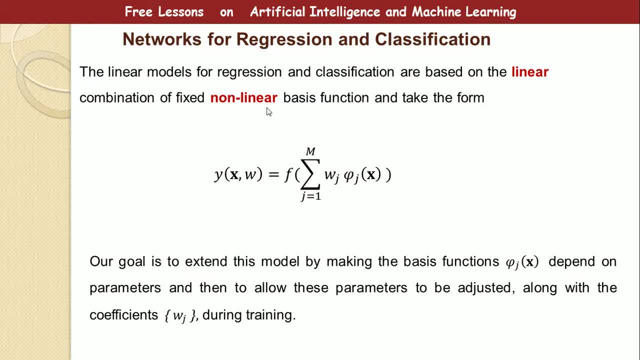 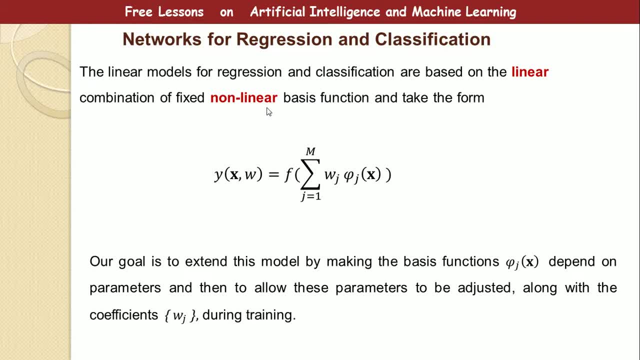 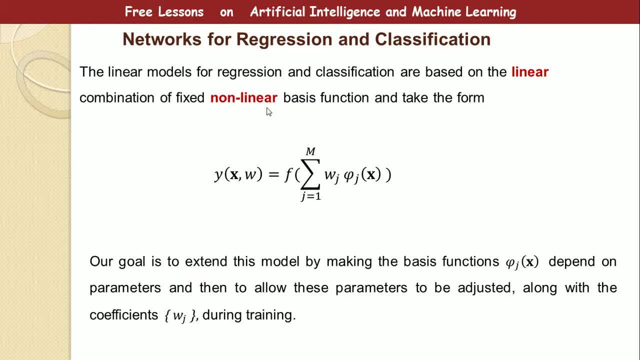 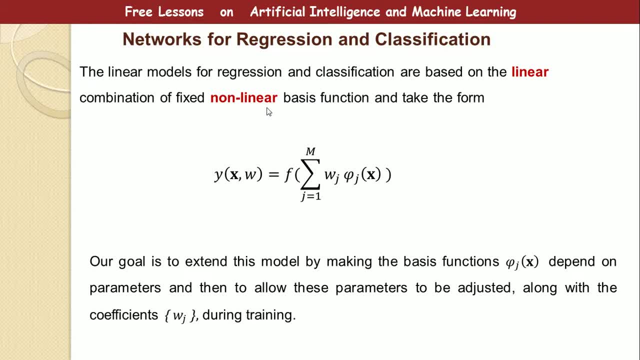 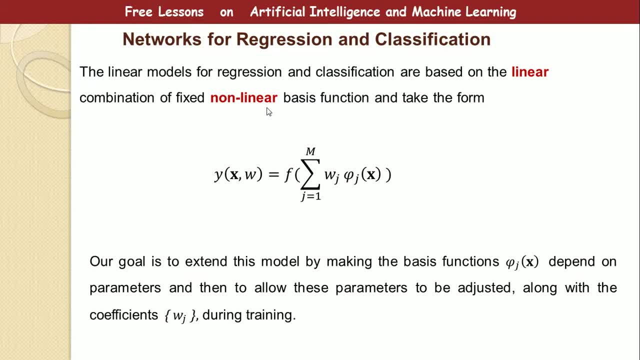 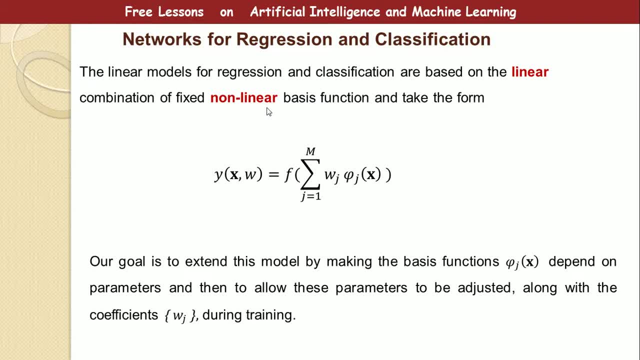 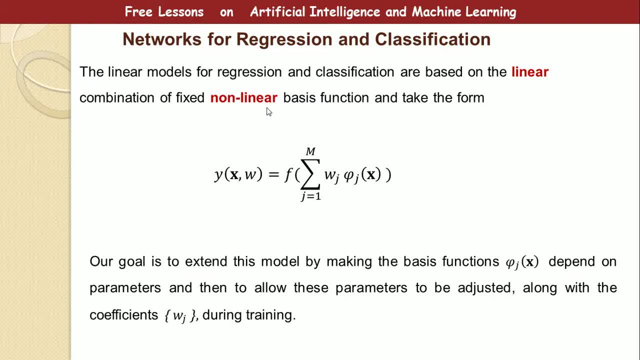 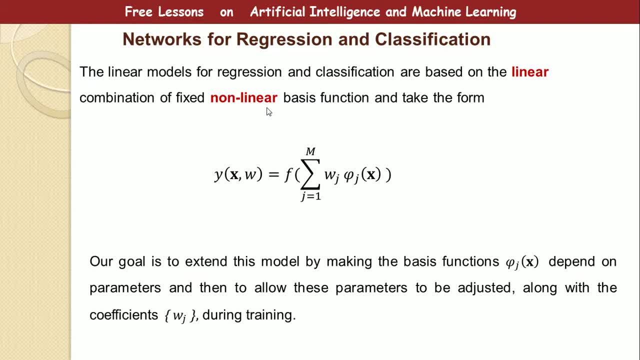 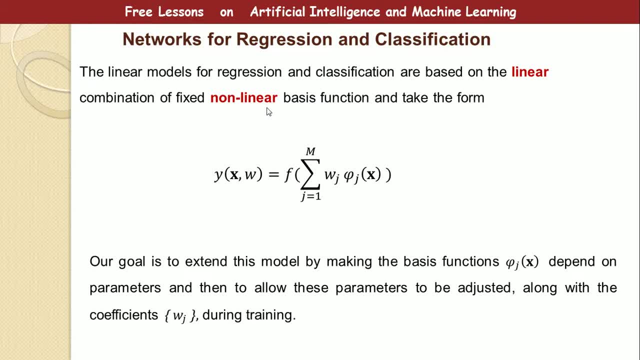 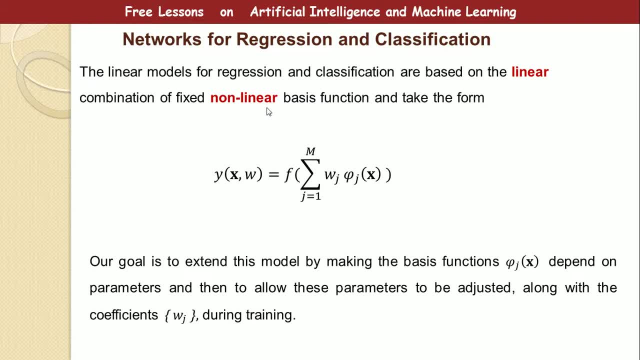 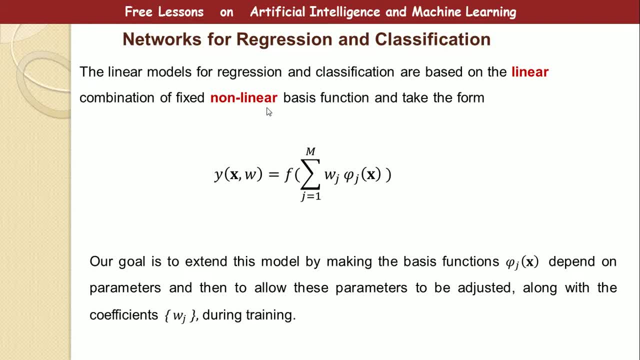 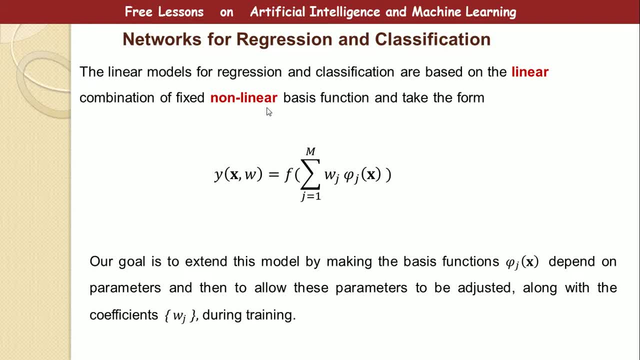 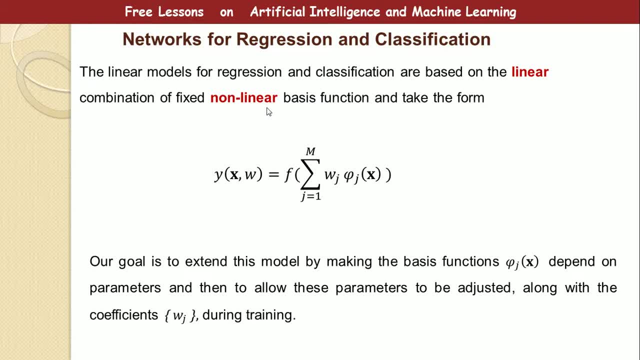 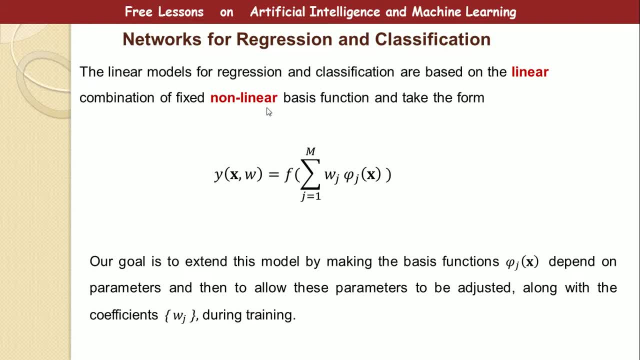 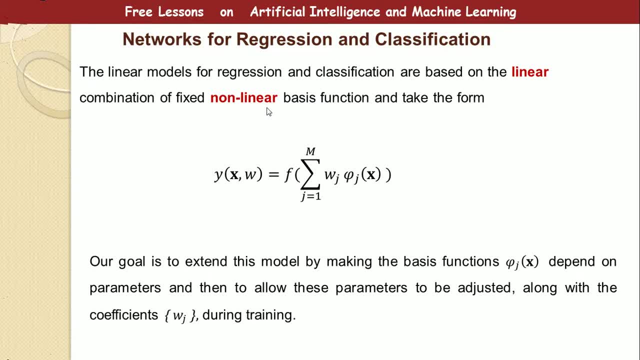 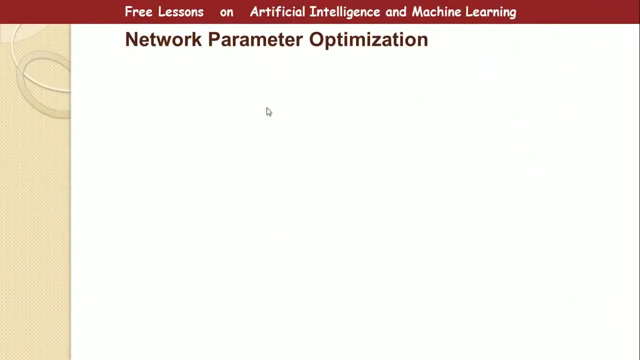 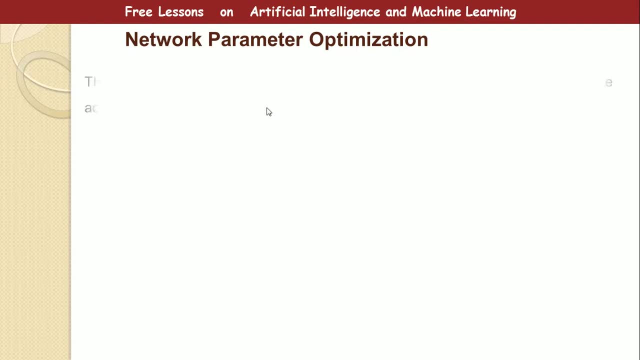 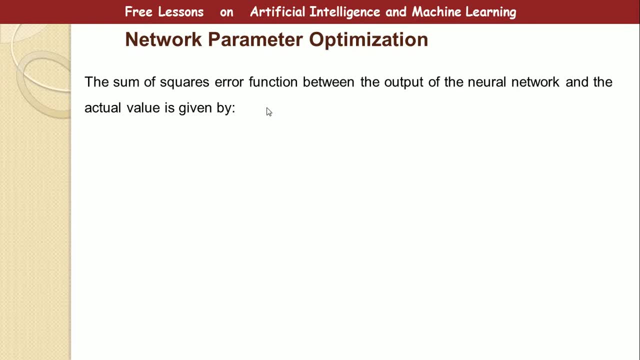 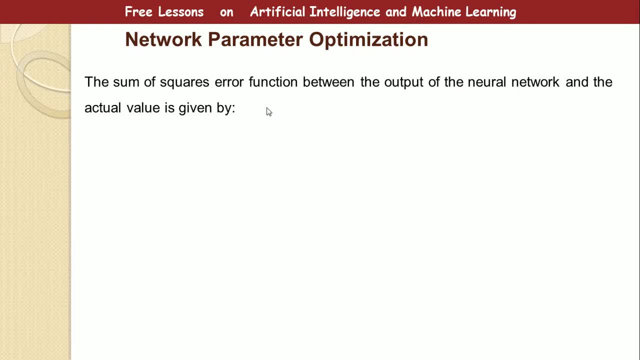 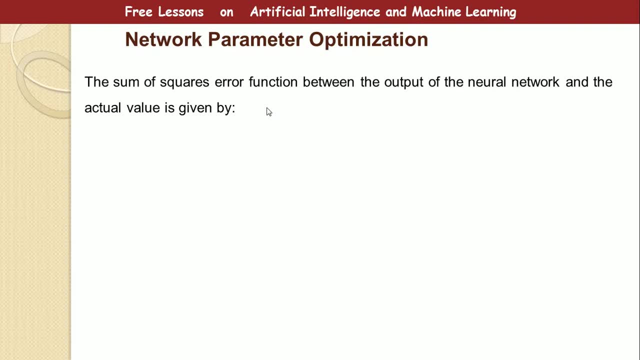 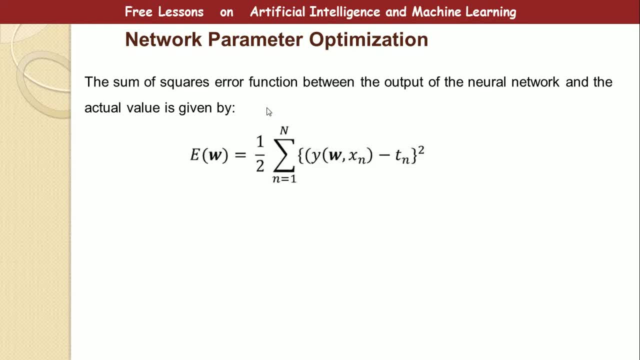 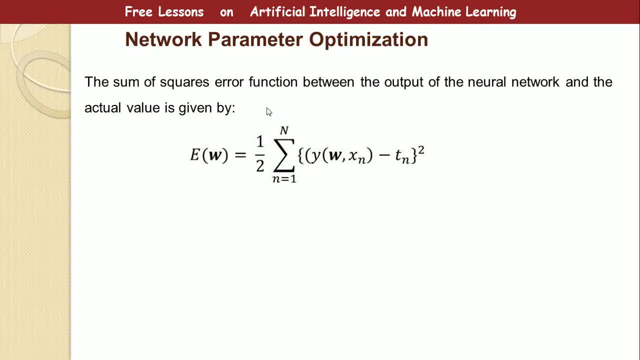 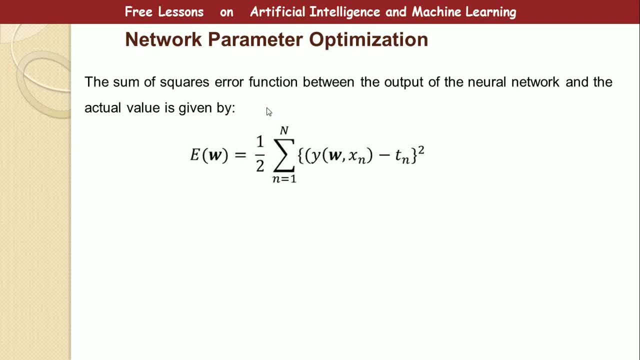 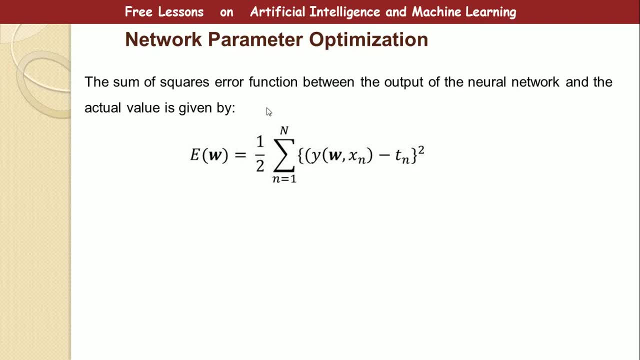 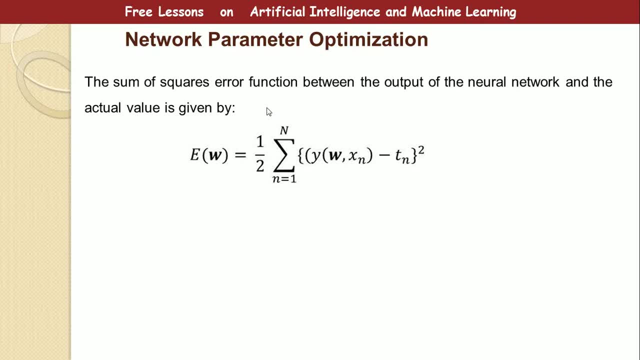 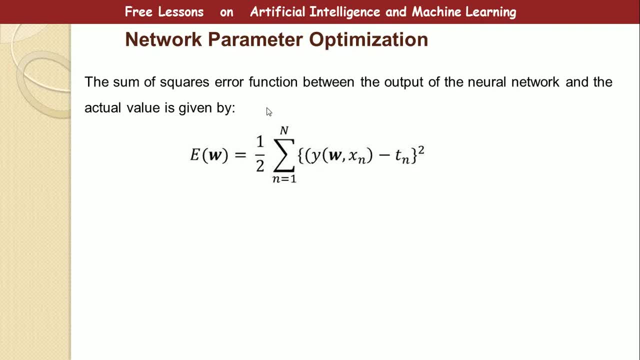 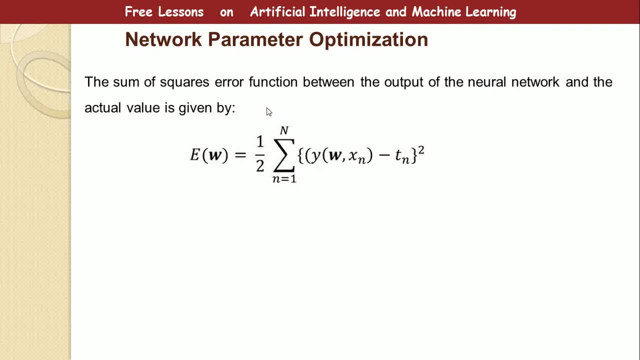 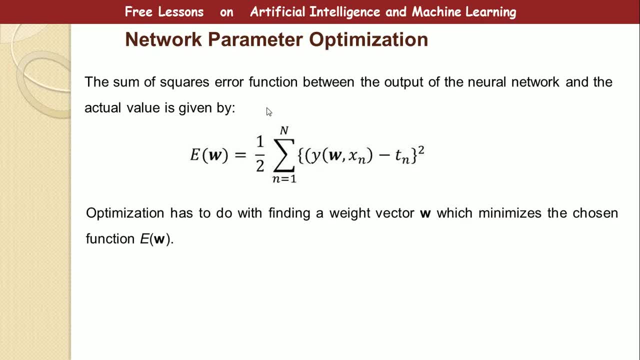 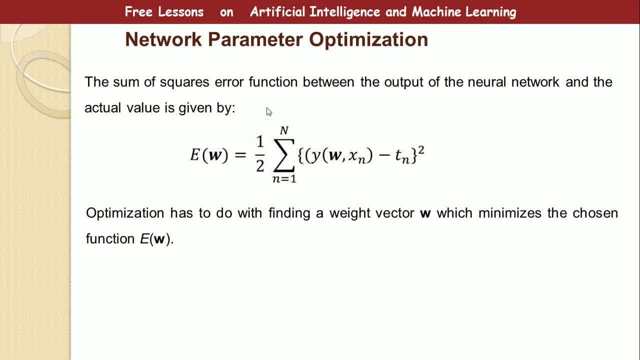 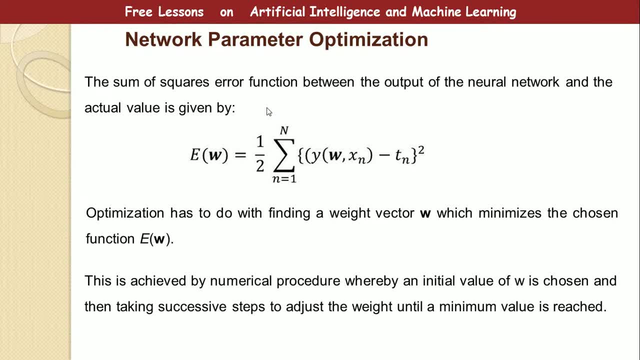 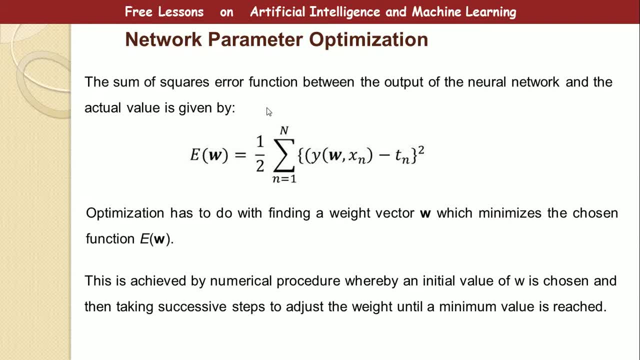 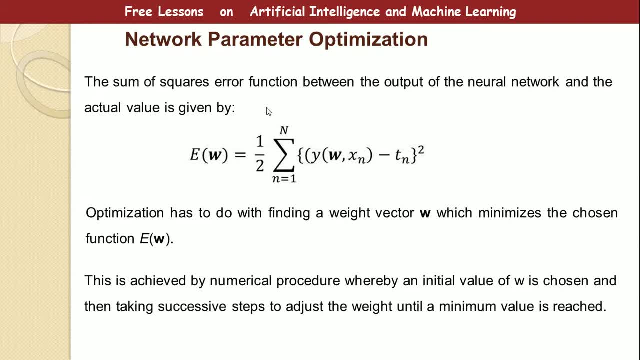 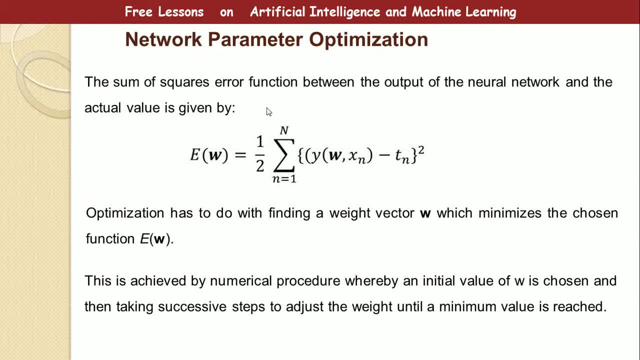 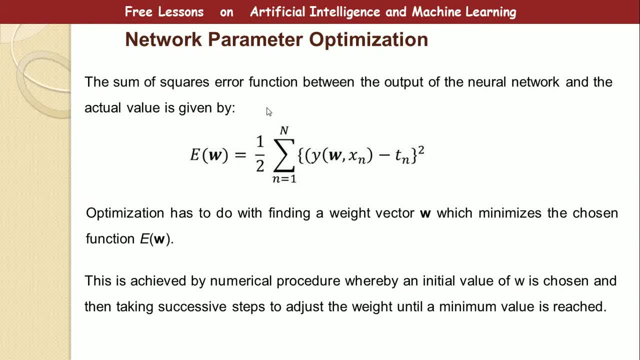 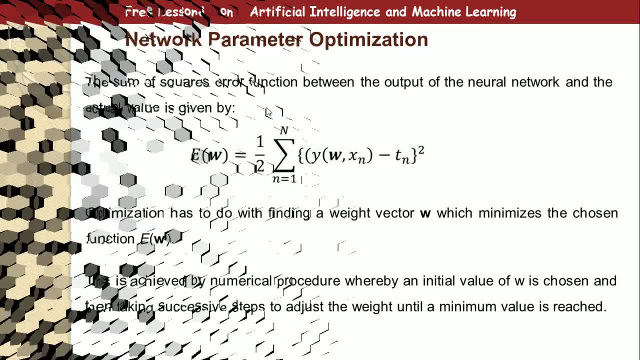 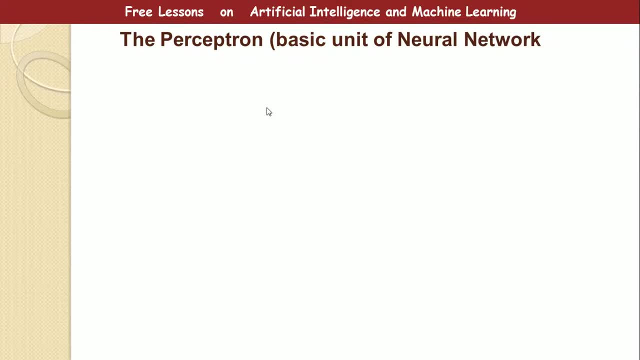 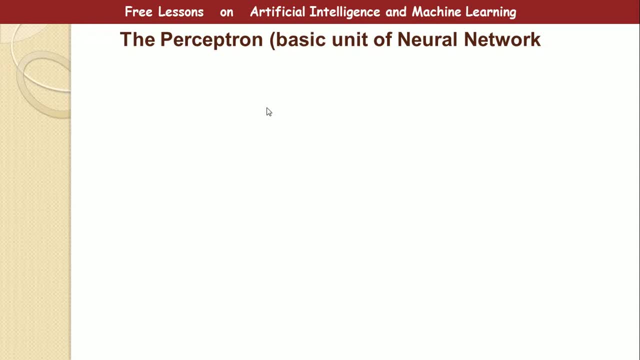 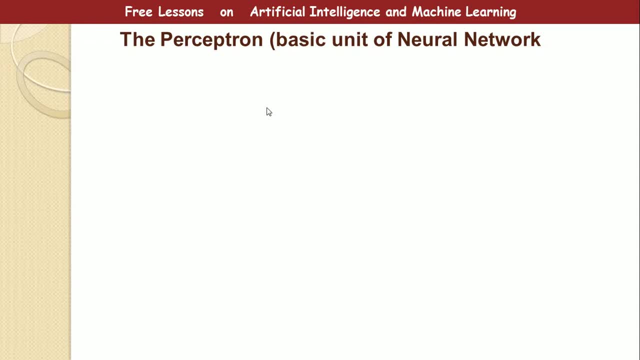 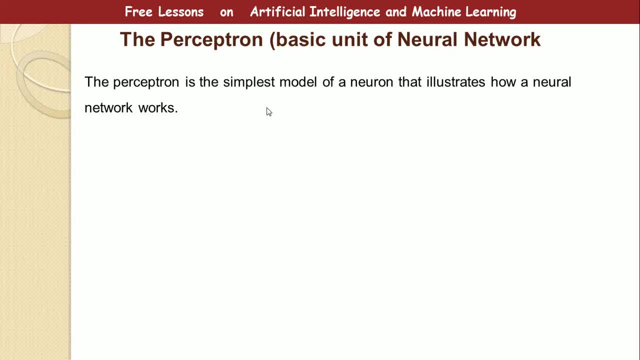 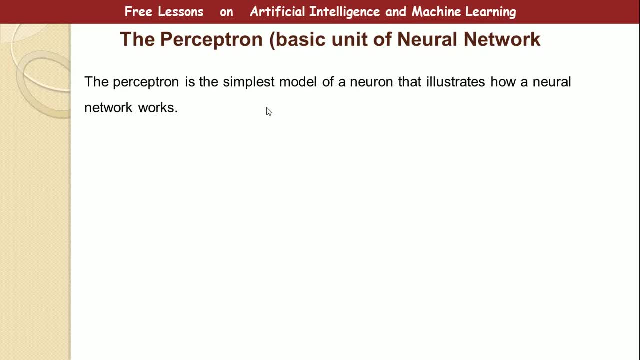 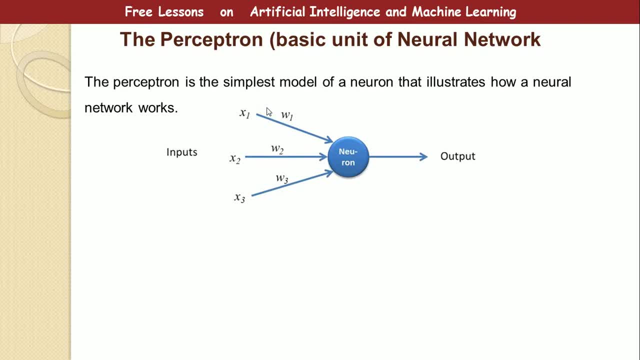 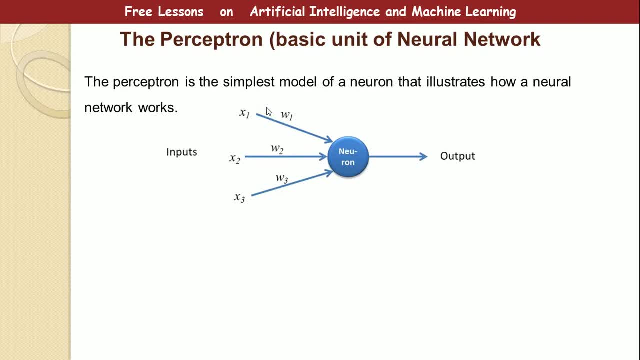 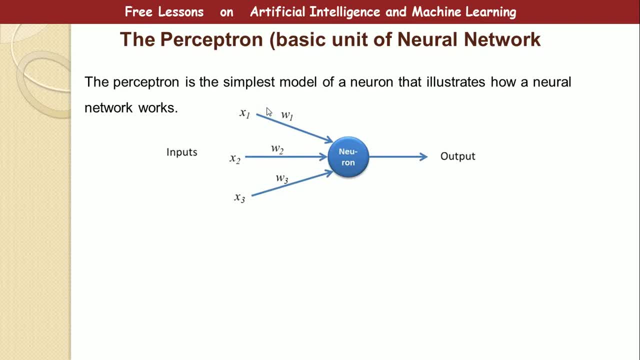 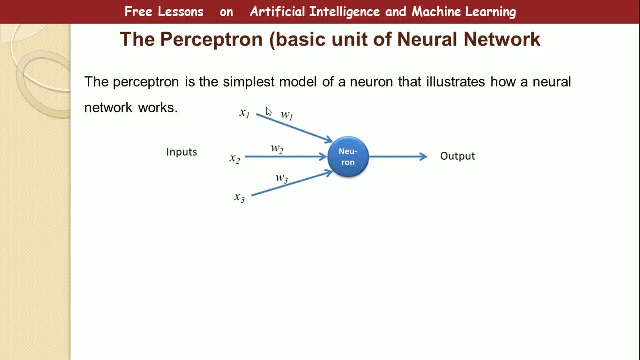 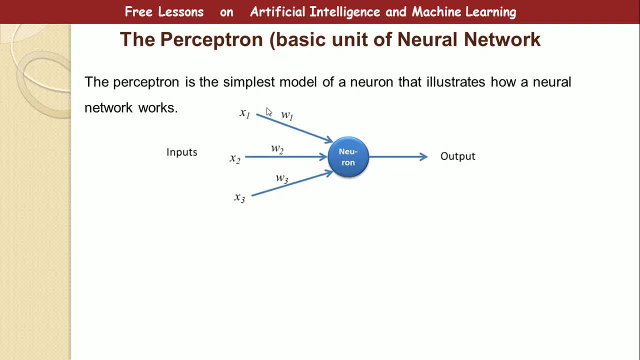 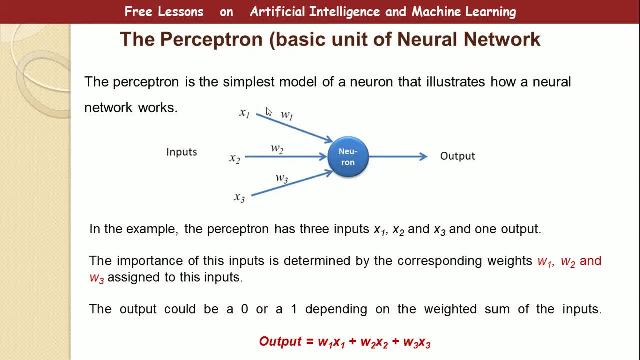 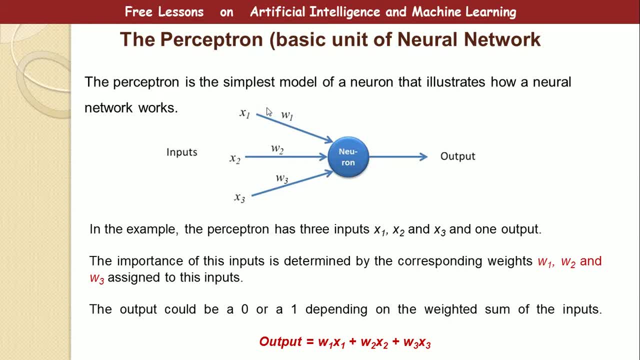 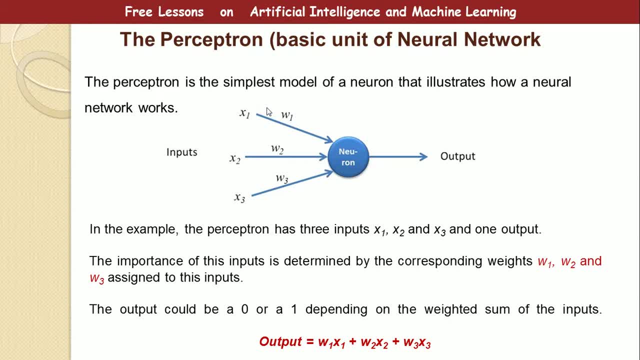 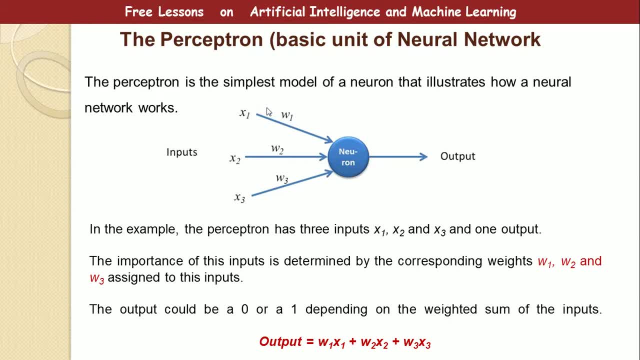 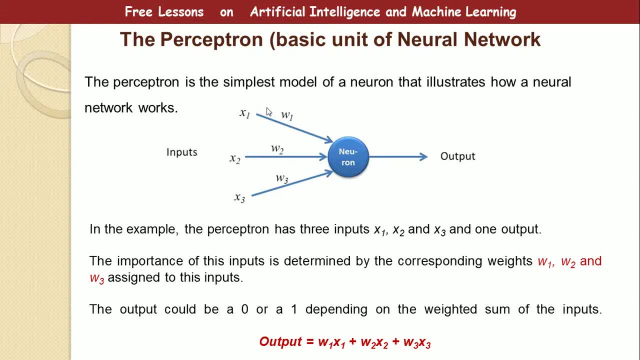 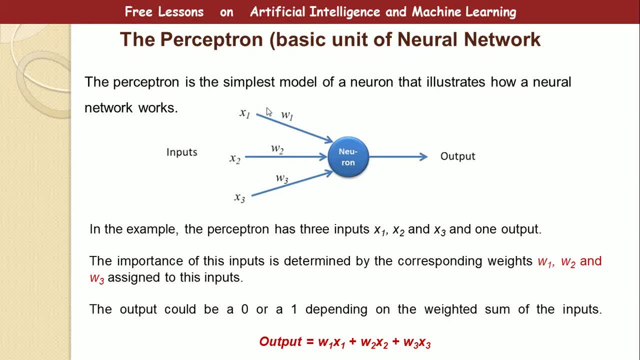 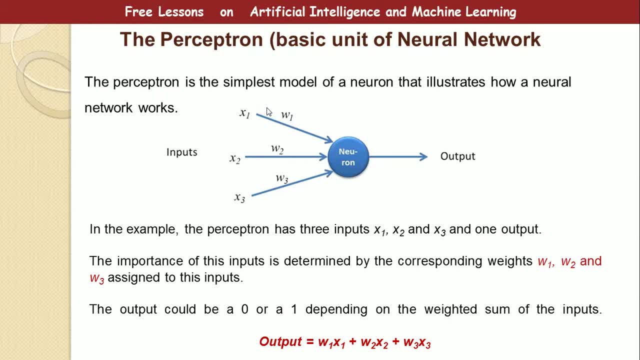 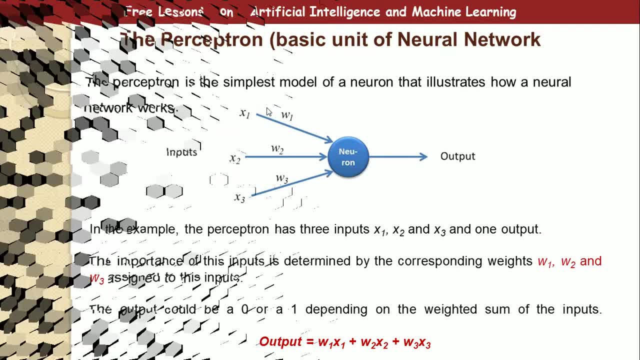 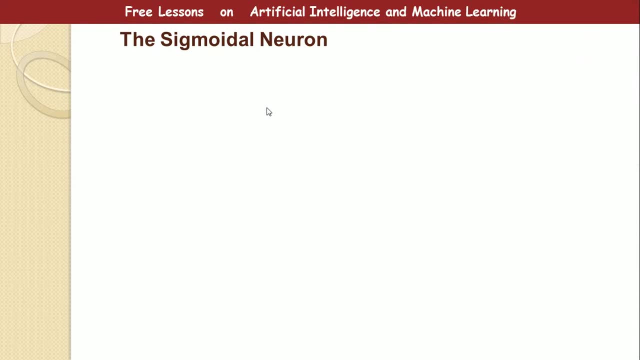 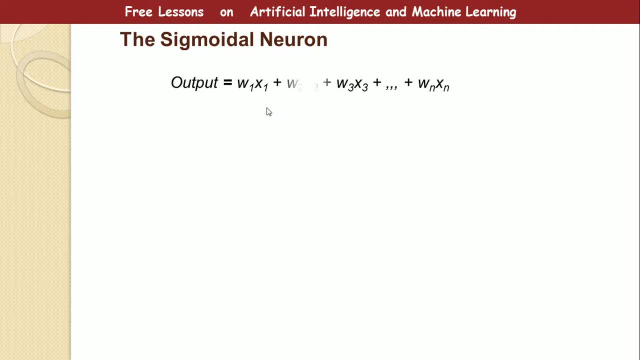 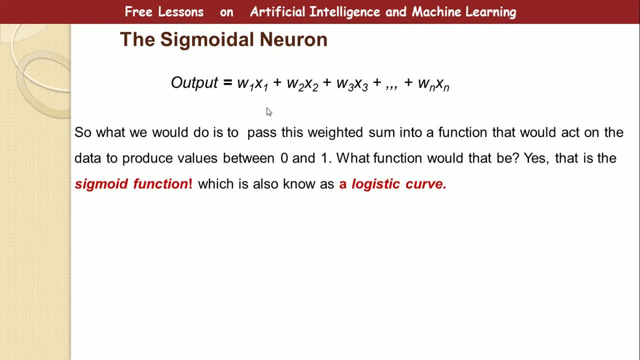 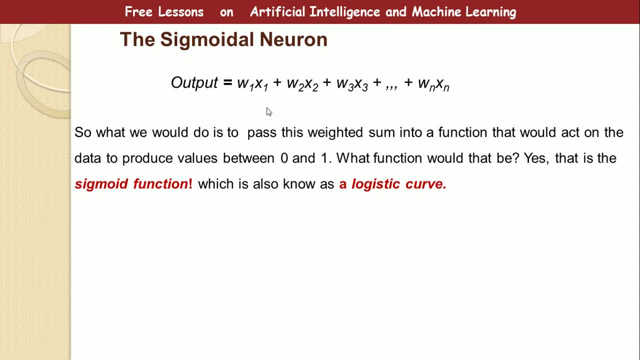 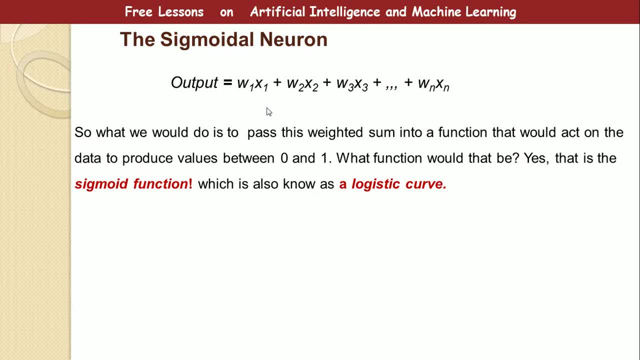 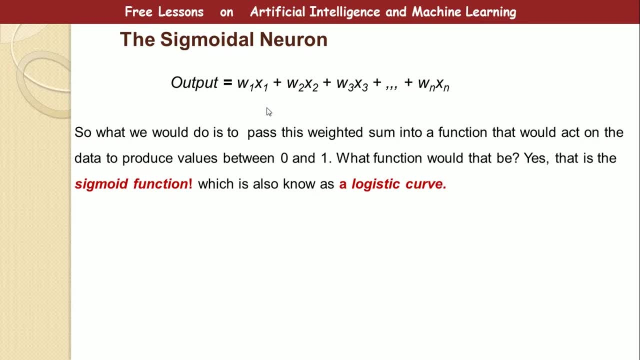 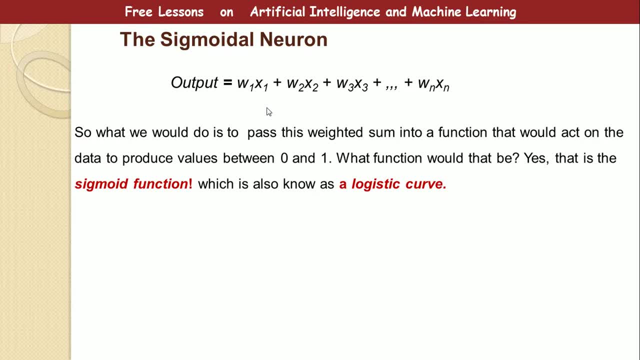 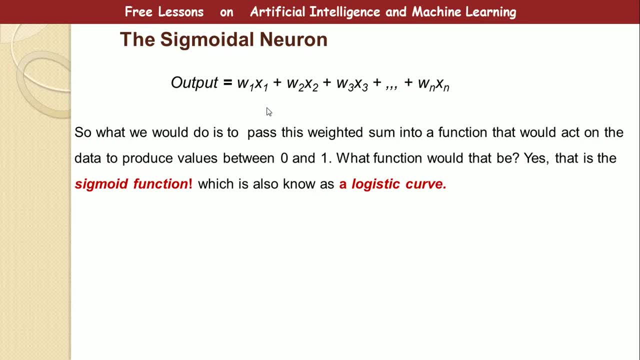 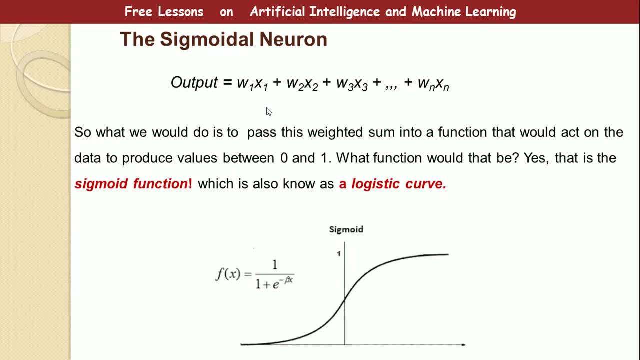 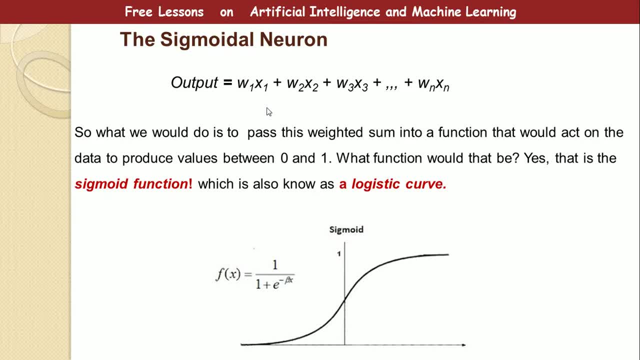 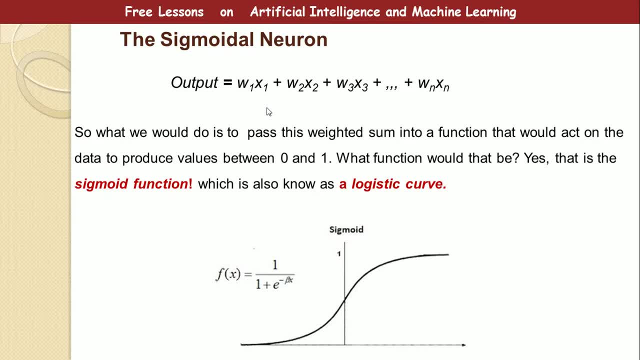 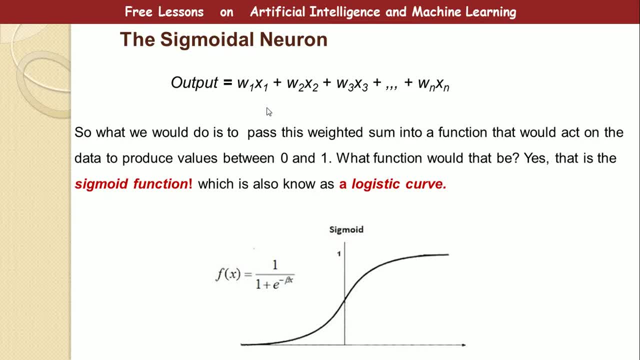 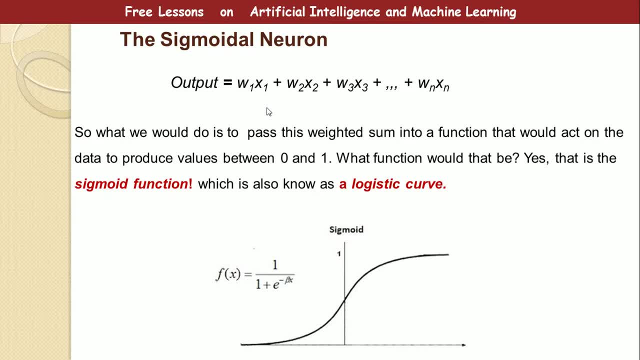 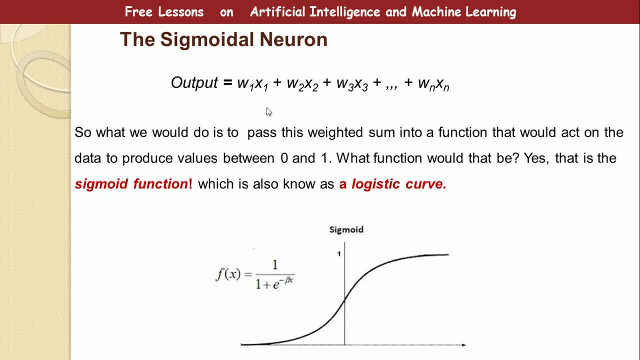 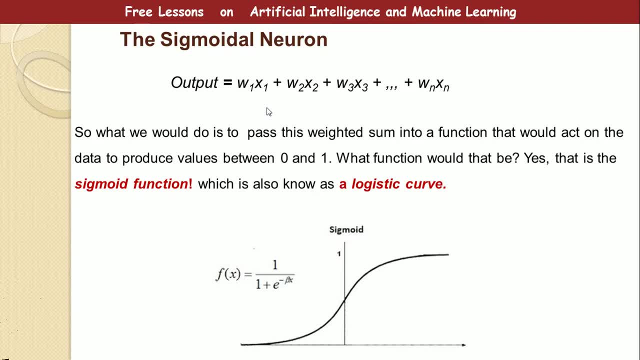 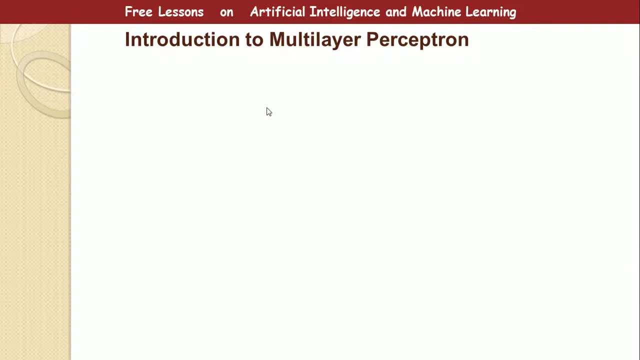 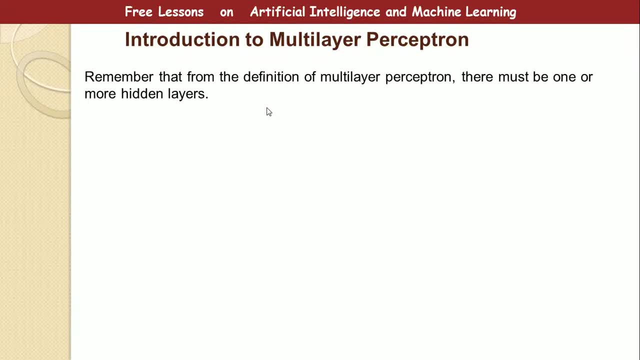 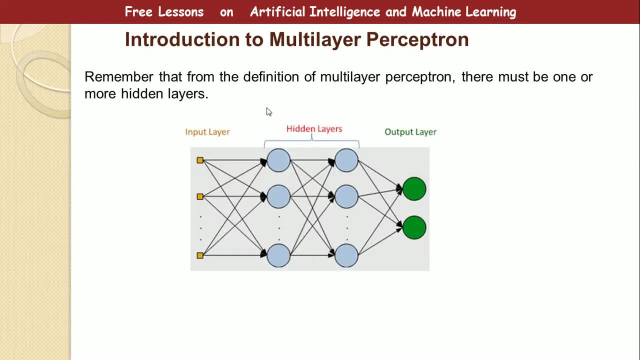 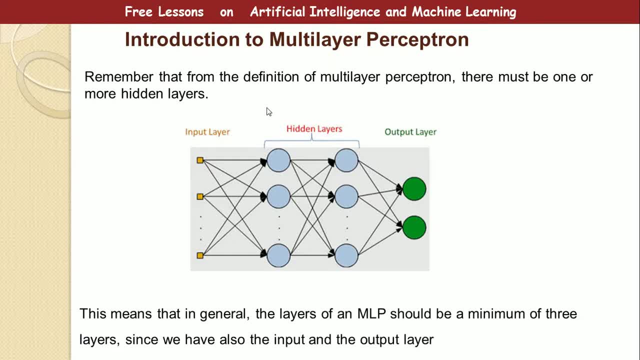 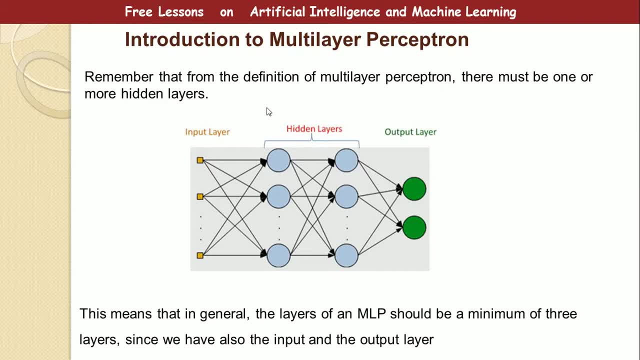 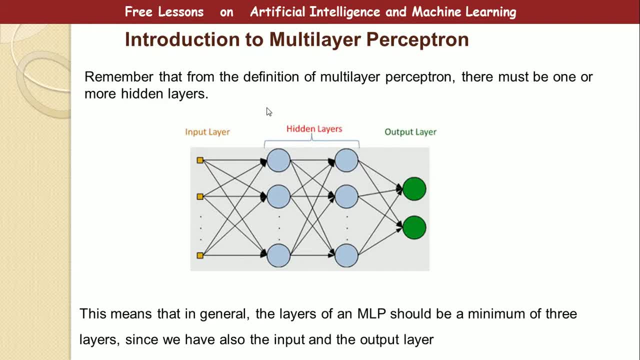 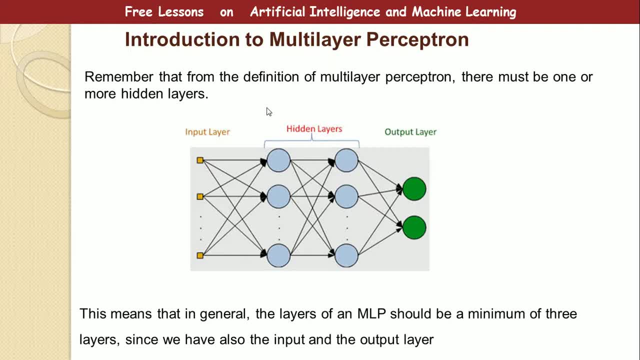 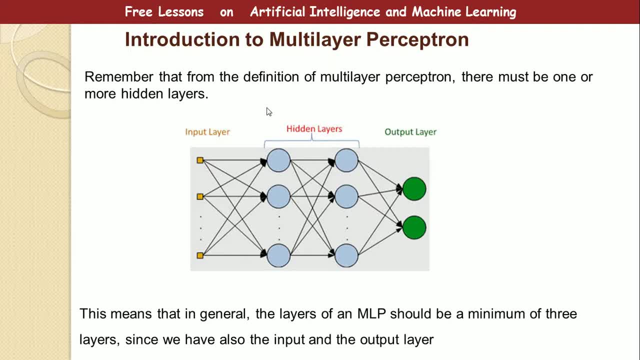 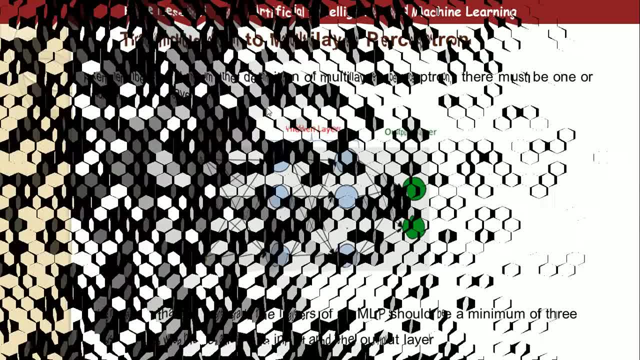 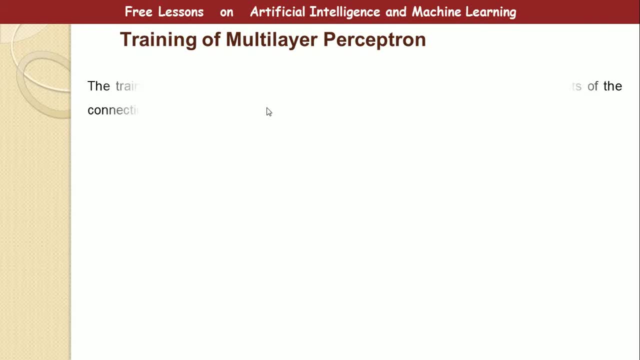 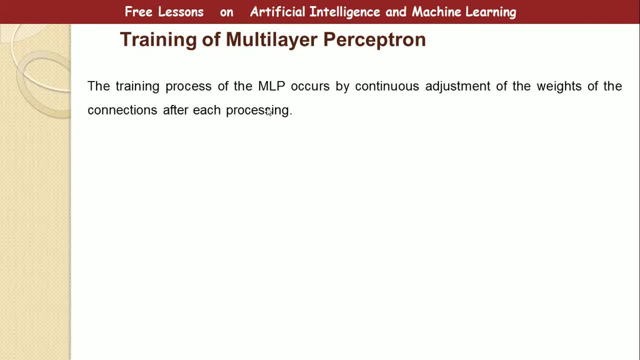 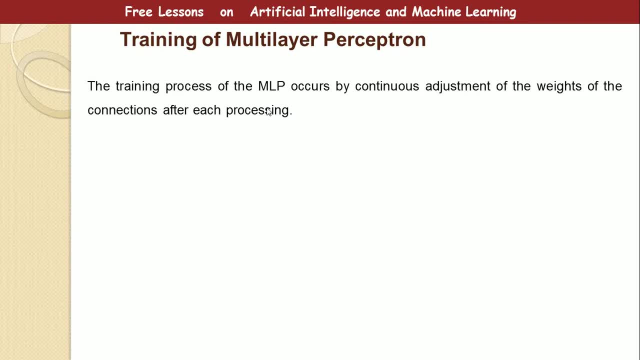 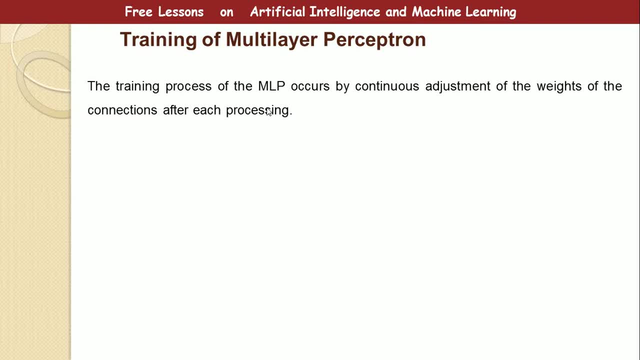 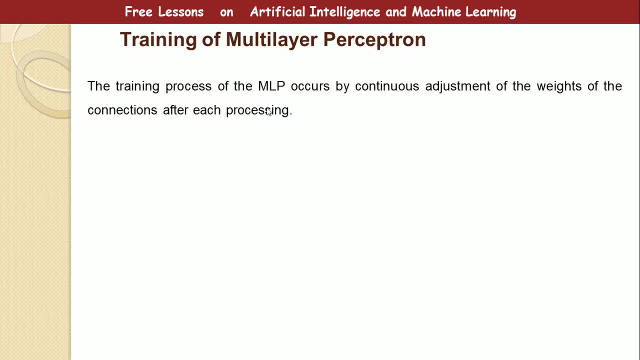 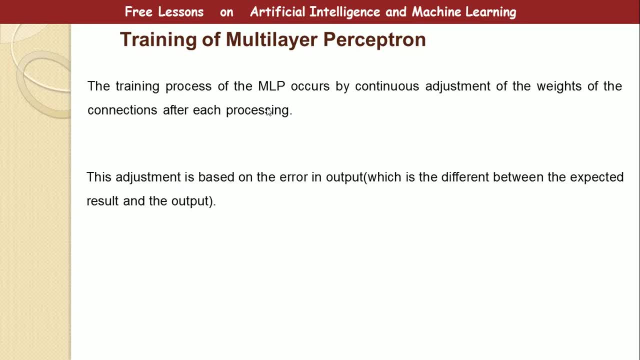 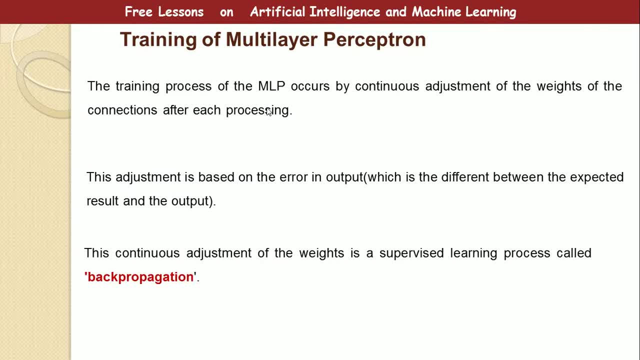 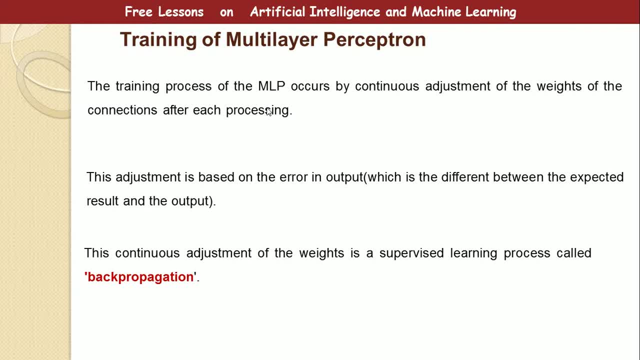 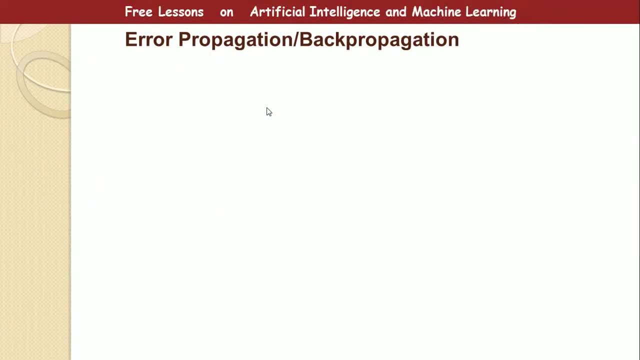 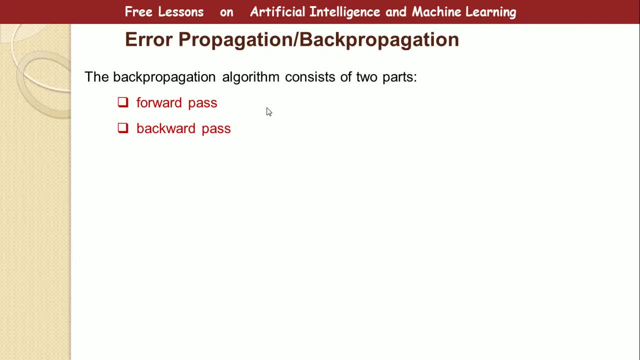 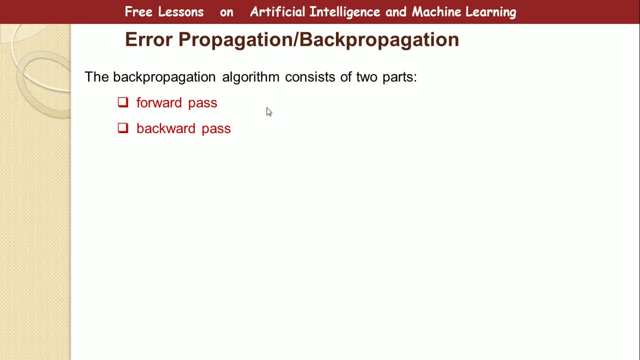 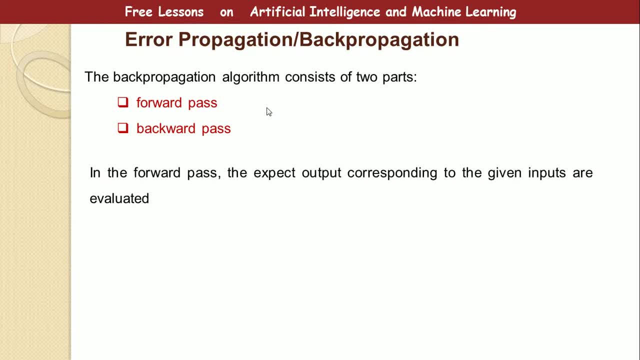 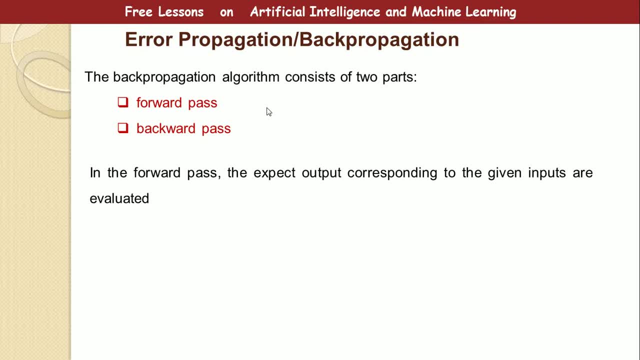 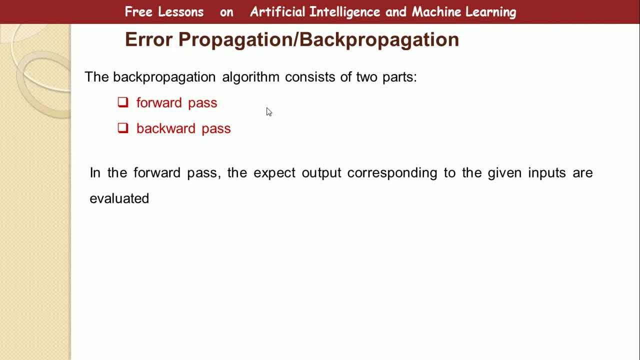 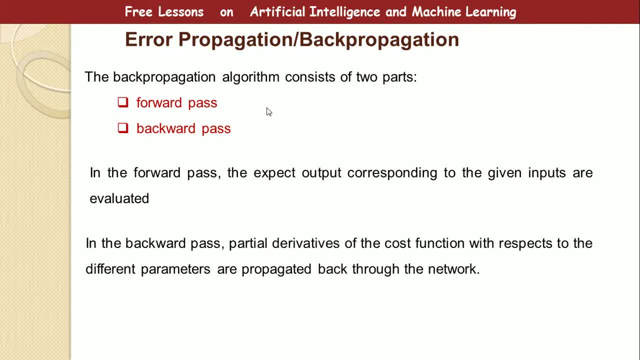 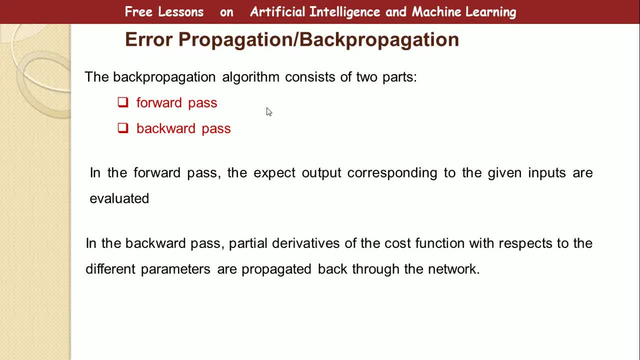 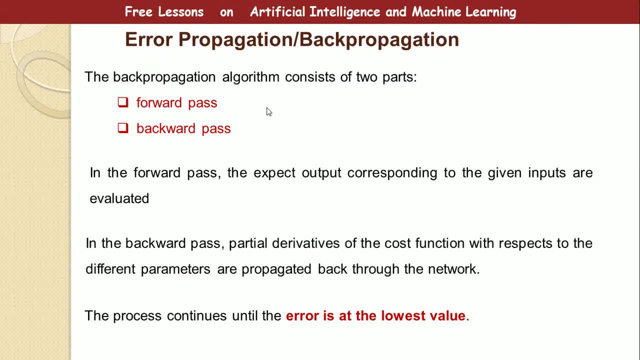 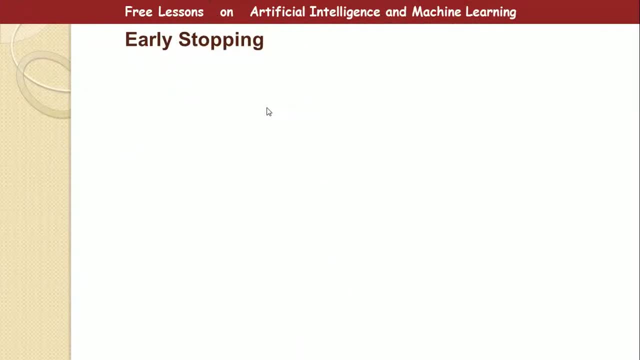 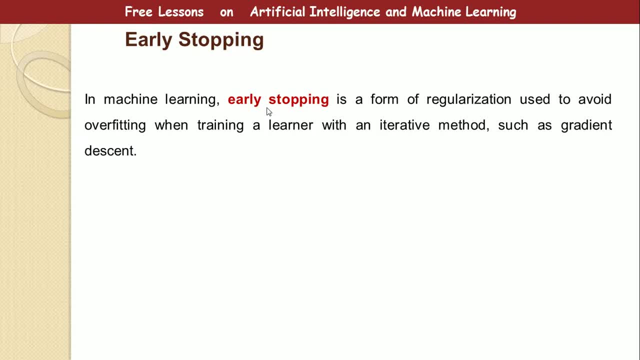 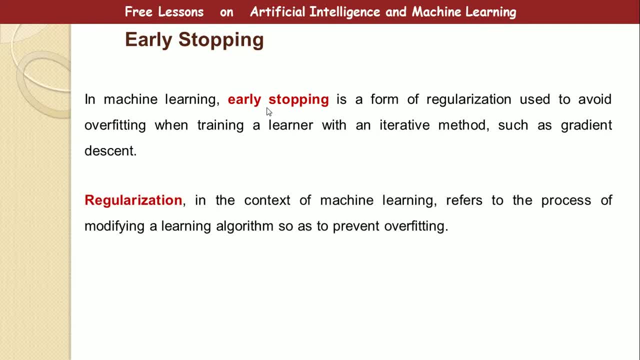 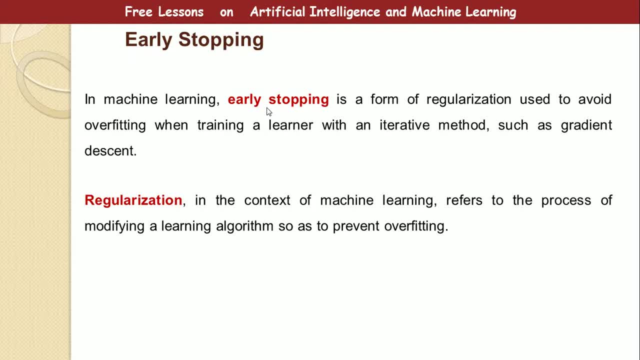 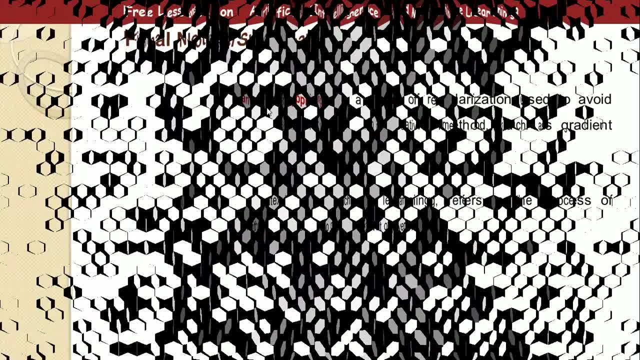 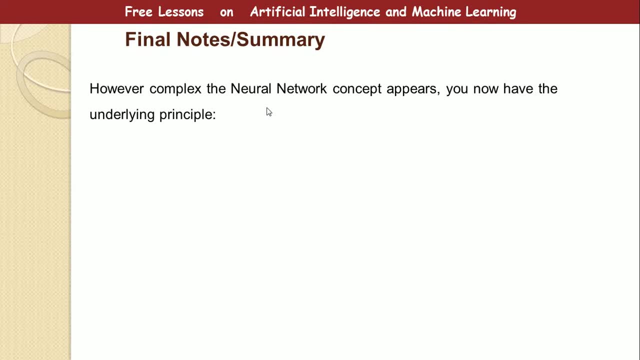 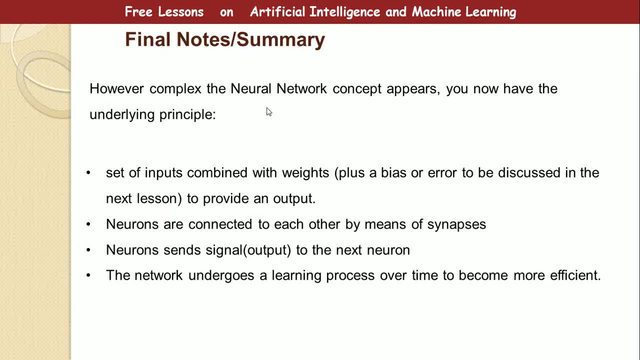 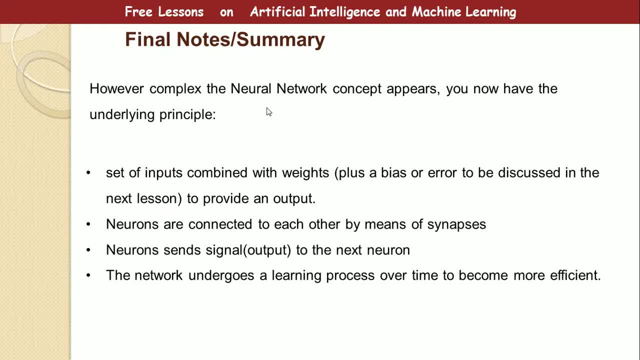 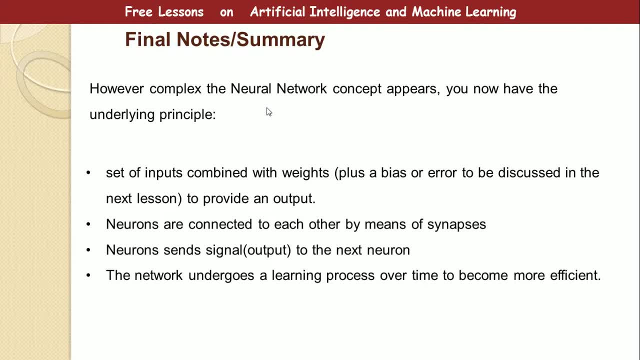 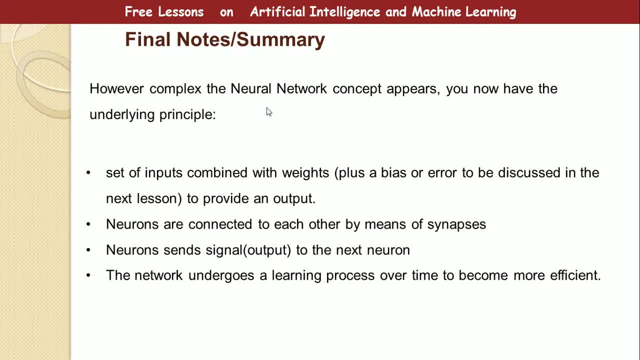 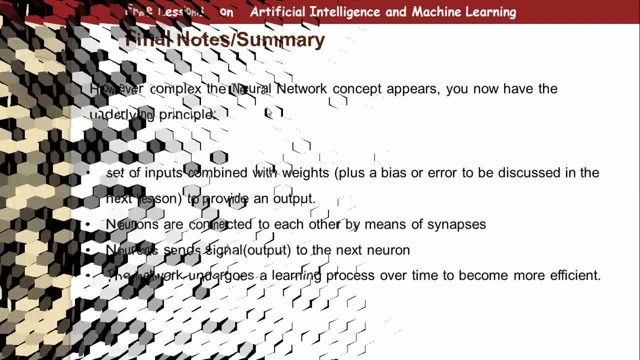 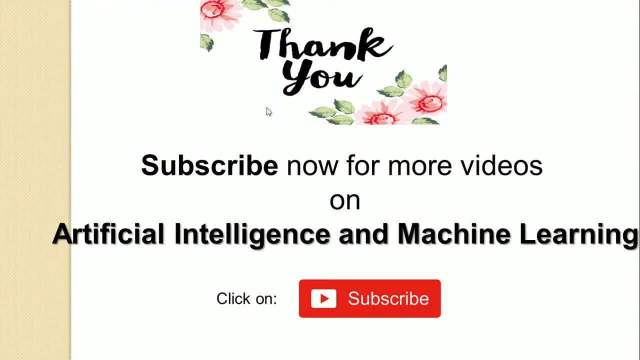 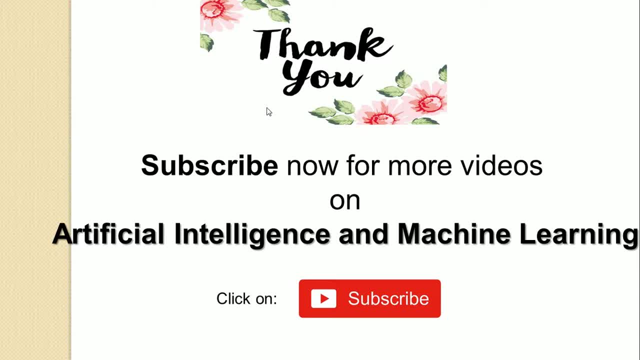 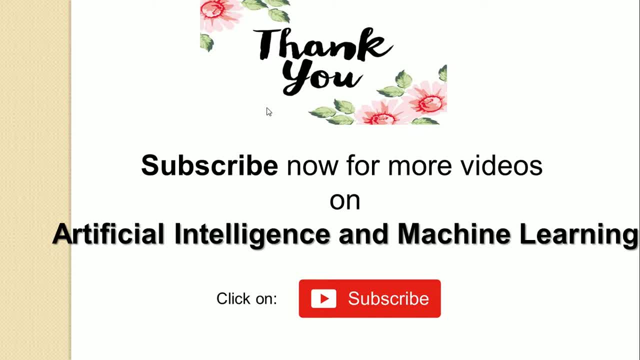 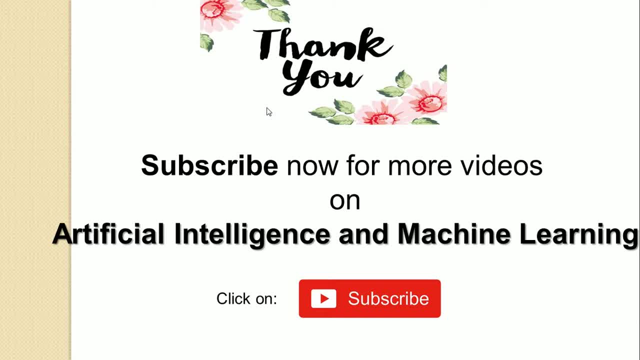 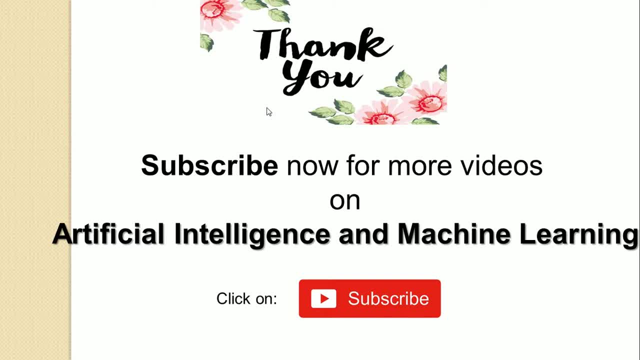 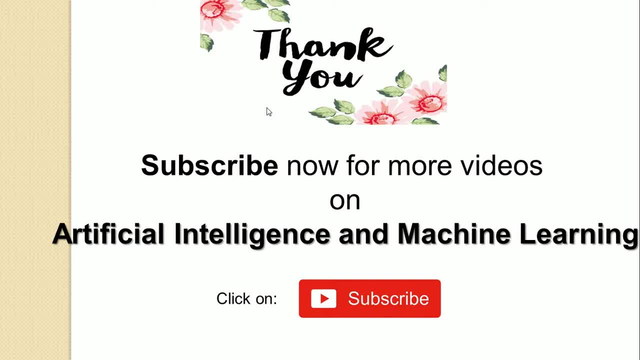 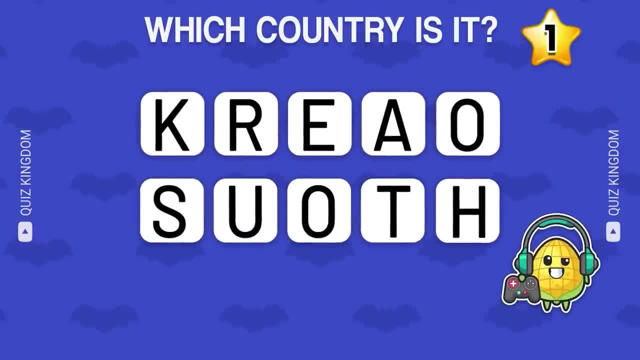 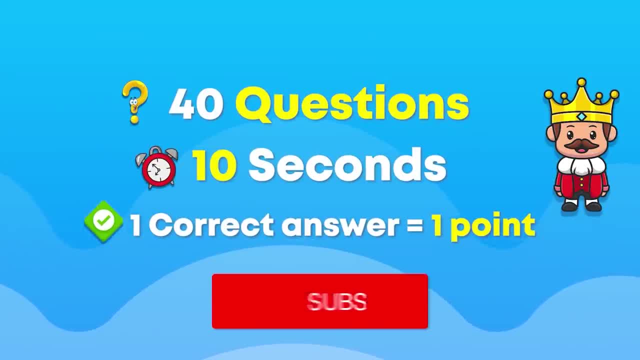 Hello everyone and welcome to Quiz Kingdom. In today's video, we'll guess the country by its scrambled name. We've prepared 40 questions and you have 10 seconds to find the answer. For each correct answer, you'll get one point. 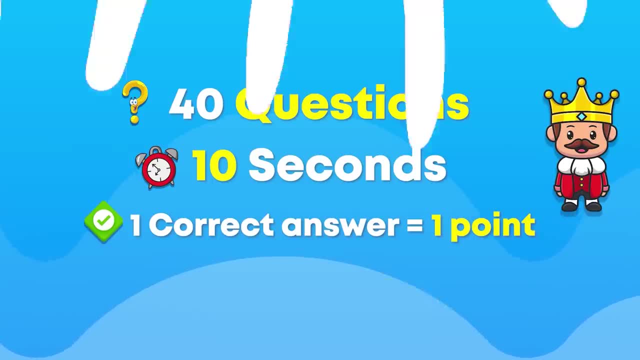 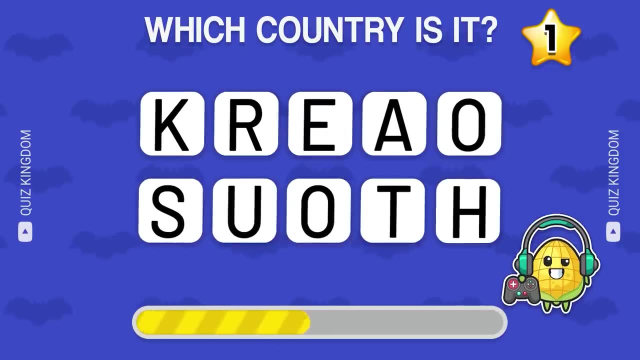 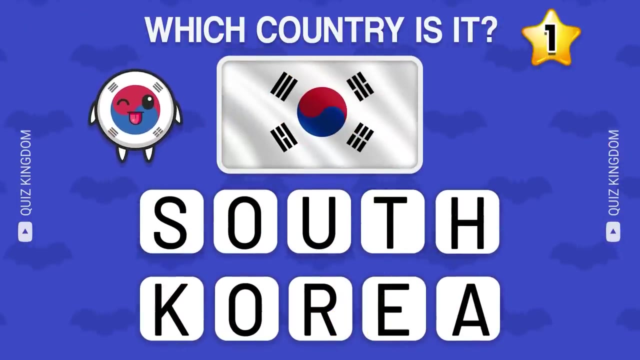 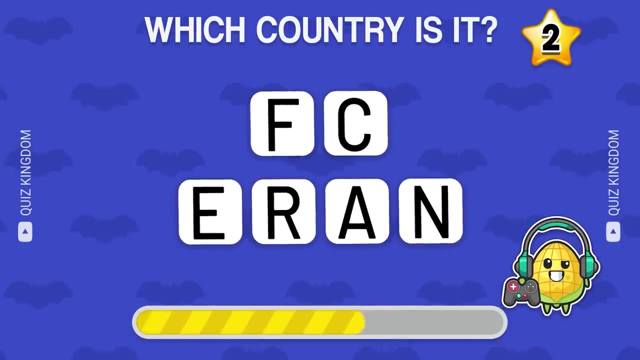 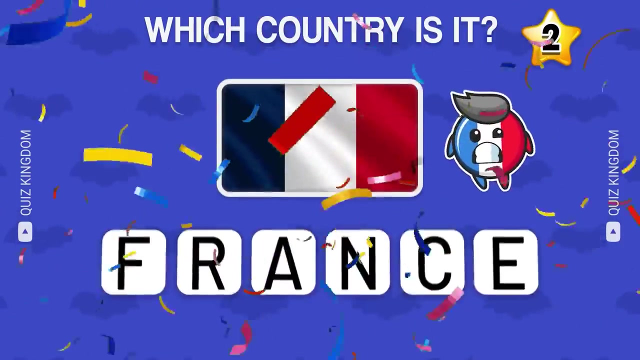 If you're ready, please subscribe to our channel and let's get started. Question 1. What country is this? That's right, it's South Korea. Question 2.: Great, the country is France. Question 3. What a long name, but I think you could do it.